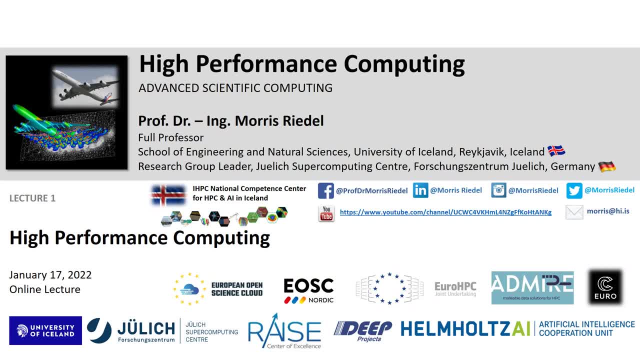 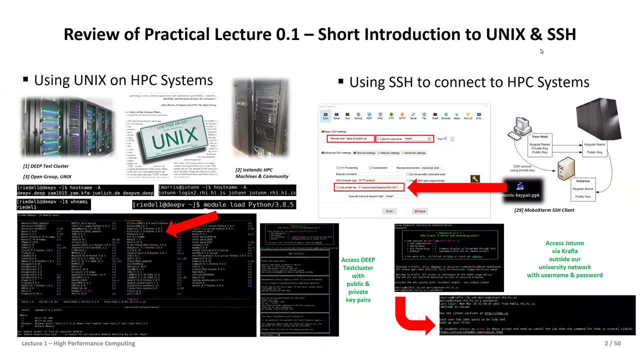 in the next subsequent lectures We'll be then more explored things like distributed memory, shared memory, what that means, how you program them. But before we go into the material of the lecture one, let us review what we did the last time, And the last time was really a practical 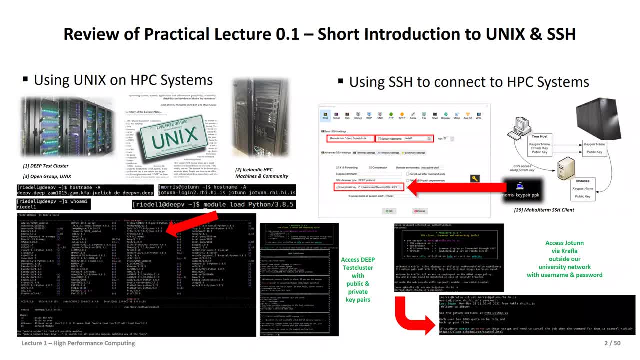 lecture which I tried to convene. you know basically all things which are more or less required from Unix. for the course There will be a bit of more commands which will be coming. really dealing with Unix in HPC is necessary if you want to work in this. 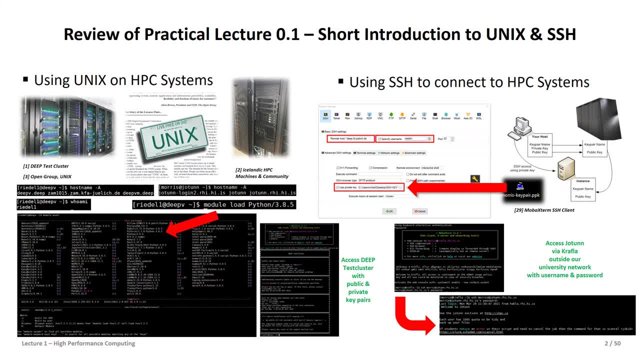 field. It's really the operating system of choice. We have seen some Windows clusters, we have seen, basically, other systems, but basically these systems require Unix knowledge in order to at least have the baseline ready. Things like creating directories, of course, we have discussed. 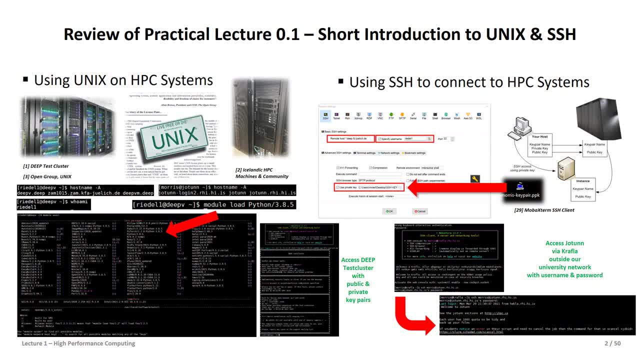 but also understanding, perhaps, here and there, the distributed nature. what you see here is host name minus A, which directly shows you that essentially we have, let's say, remote systems we connect to, but then also, of course, dealing with the idea of the module environment. 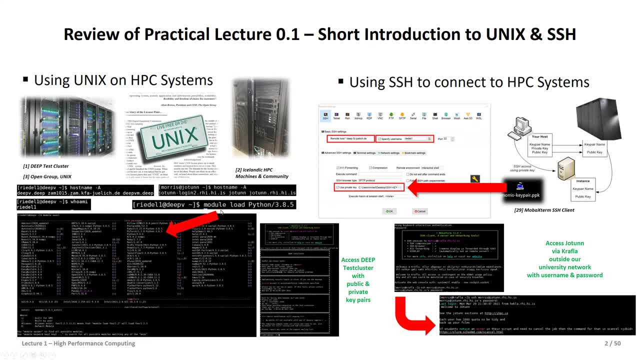 that we learned last time, where we basically said: like there are lots of pre-installed software here already available on these supercomputers And there's a so-called module environment where you can module, load specific modules like the Python and a specific version here. 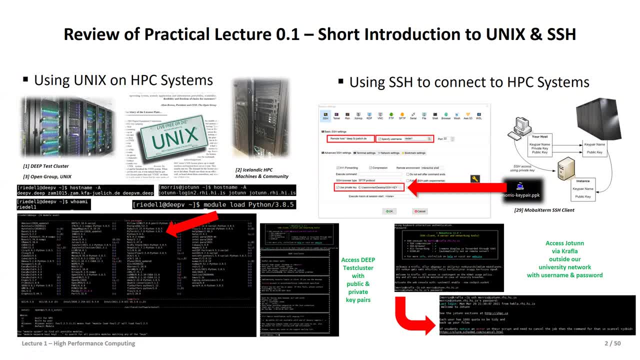 And the benefit was really: we have different, let's say, versions of A label. Now, this is another software and it's basically available directly via Unix commands. So you have module avail module, spider, module, load. but this again shows you why Unix commands. 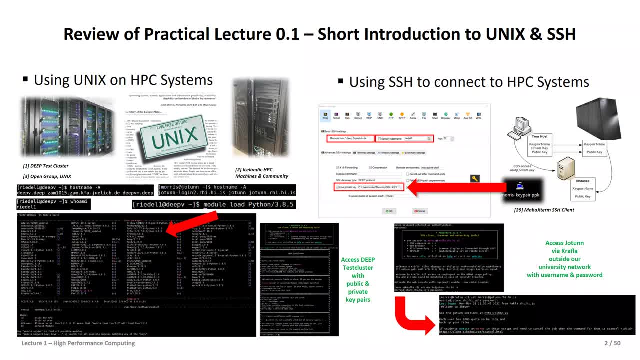 are so important to understand. Of course, if you're using basic Unix, like I say here- like who am I- that gives you also an interesting insight of what is your real login. By the time you're logged into the system, usually you should know your username. 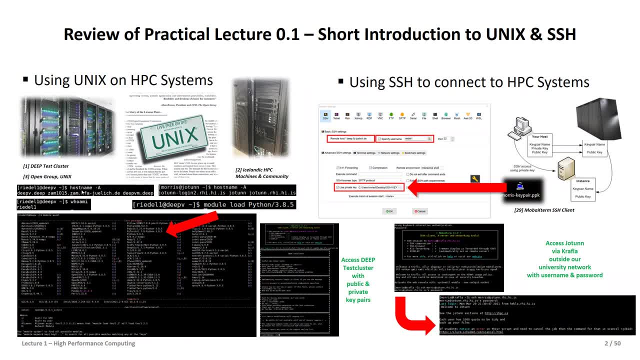 and you should know the host name, and why is that so? So, basically, these are the two key requirements that you need to know in order to basically log into a system, as we call it. We talked already that these systems let it be the deep. 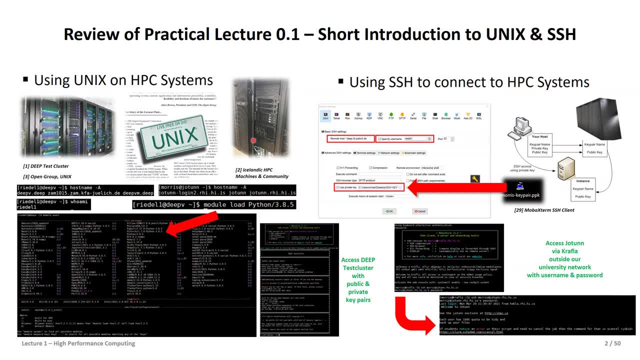 test cluster that we're gonna use in the course, or our U-turn teaching cluster are remote systems. They're not your laptop machines. They are basically accessible via the internet here and there, only via the internet of the university or so, but still they are remote. 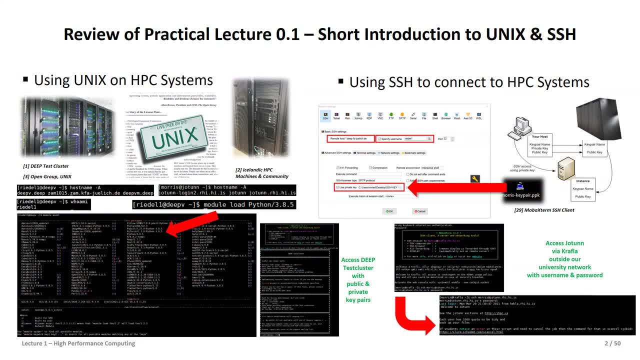 and you have to log into the systems. A login requires your username. And then, of course, the other aspect is it, which is a direct URI you want to basically go into, You want to basically connect to, And for this we have used the so-called secure shell protocol. 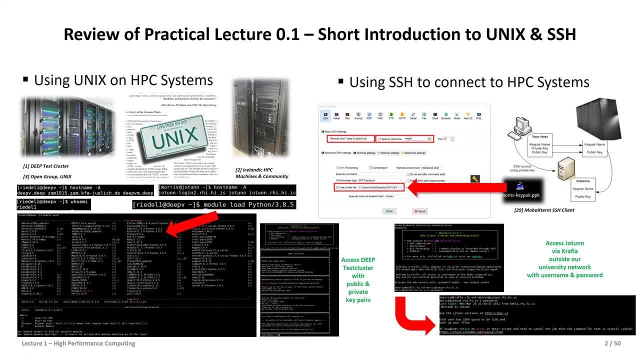 where we can log into another HPC system which is away from my laptop, And I can use two different principles. We'd have that done last time And I showed you some demonstrations how that really works. where the one was really then our deep test cluster. 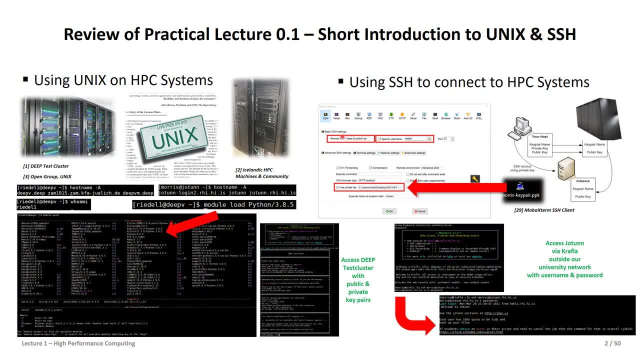 where essentially, you have a specific remote host that you put in in the system And then you have a specific SSH client that you see here. This was the example of the mobile Xterm client, but you can use any other SSH client like Putty. 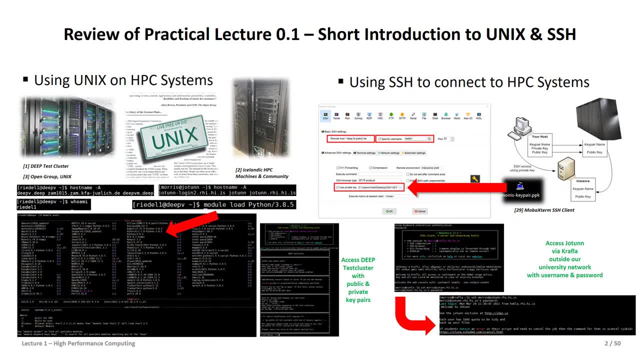 or Unix derivatives. Of course, if you drive a Linux somewhere, you can also use a command line for the SSH. It really doesn't matter. What much more matters is that you know your specific username and the specific host name, And basically these systems have different policies. 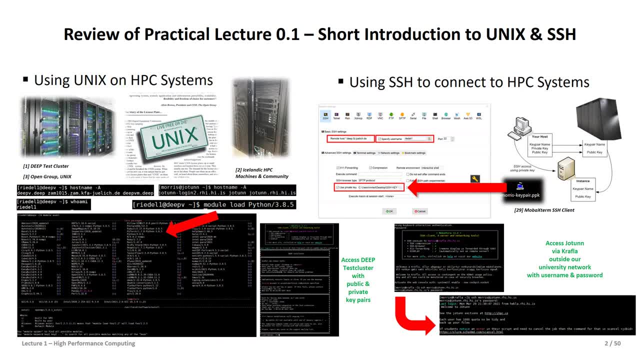 when it comes to all of this. So you can use the SSH client, but you can't use the mobile Xterm client. So that's one of the things that we need to do. And then the other thing is the authorization, authentication and so on of users. 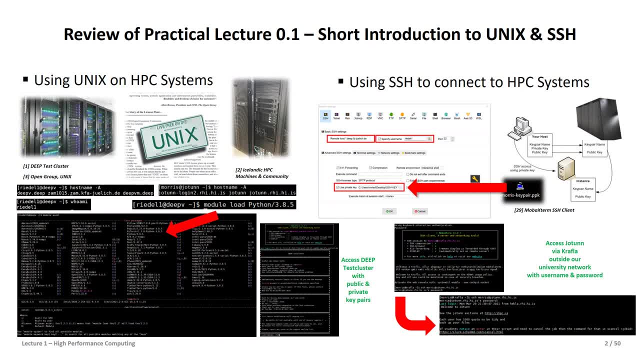 And this particular one where we said the deep test system, is very similar, like many HP systems worldwide which are in operation and production. Production means really users use it every day for scientific and engineering problems to simulations for AI. But the key essence to take away is really: 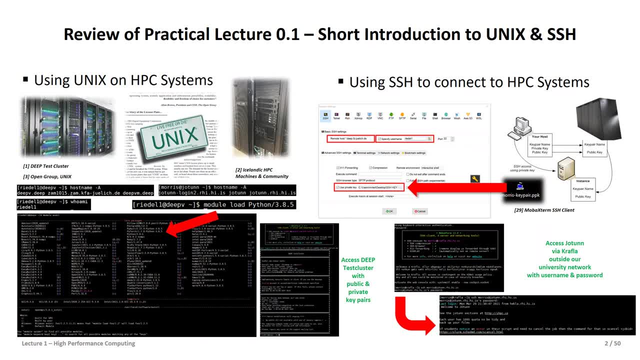 those systems are always protected with a private public key pair usually. So you would find very rare systems outside in the field in HPC which are just accessible by username password. So the SSH key principles here basically based on RSA, this public private key pairs we discussed last time. 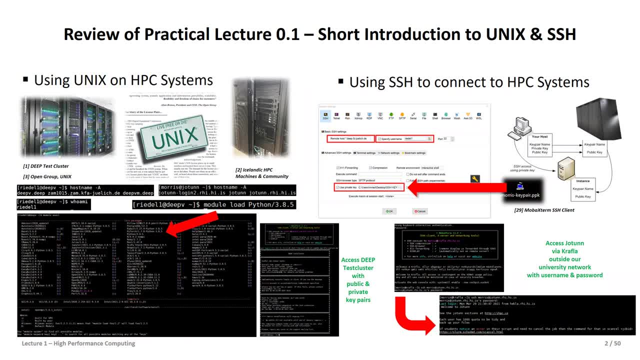 is a very fundamental approach that you basically will see when you use any other system in Jülich, in Barcelona, in America, in China. they all have these basically approach And how it works. we discussed last time a little bit. So you would have a private, public key pair. 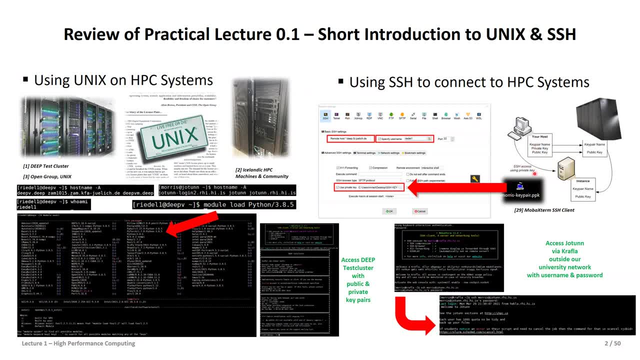 we already discussed, And important is that you never give the private key away. It should always remain on your server or on your laptop, While the public key you basically upload, and some of you have already done the assignment, so you update, maybe Udor and upload your public key there. 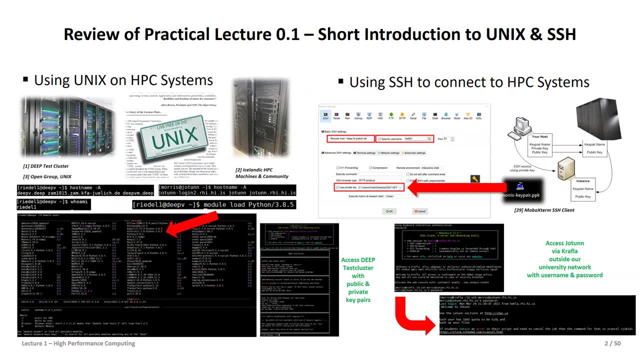 in order to get access to the deep test cluster. This is no harm. The public key is basically useless. It's useless. It's your public information. You can basically upload it, no problem. But this only works, of course, if you. 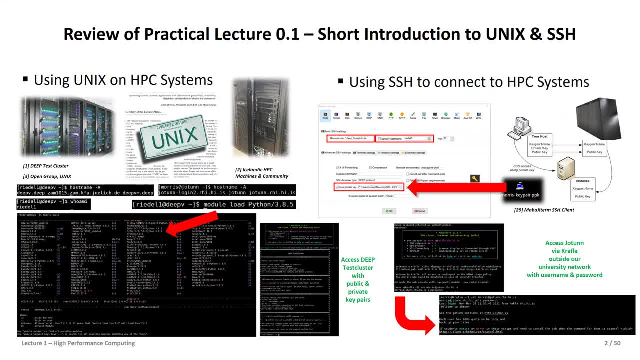 have the matching private key And there this is sensitive information. The private key should not and never be uploaded anywhere. It should be not given to your best friend, to your research group as a professor, so don't give it to all your different students. 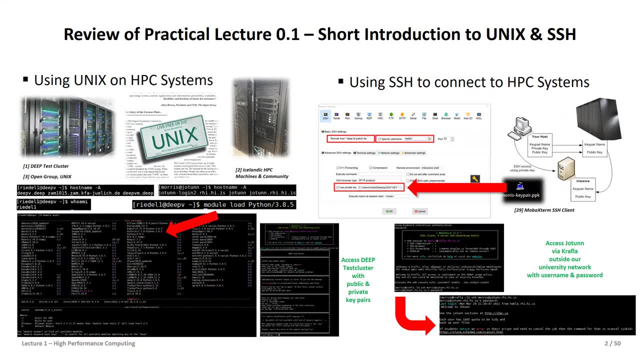 Here the key ideas. of course, it reminds your only private key And the only way how to access them- these systems protected by keys- is usually that the public key is then basically checked during the connection set up with your private key. 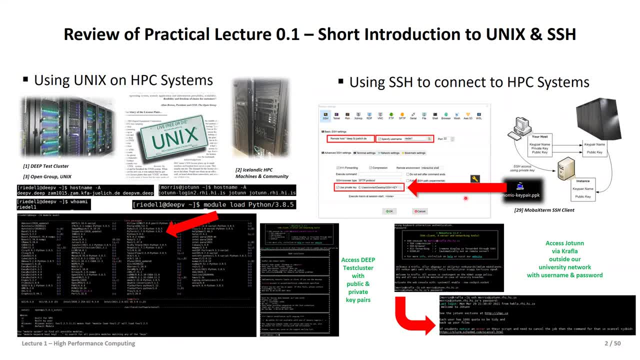 And only if that matches you are allowed to get in. There's usually no workaround that works in terms of trying three times and then get a username, access with a password or so. Usually that's not the case. You'd rather actually put on a blacklist. 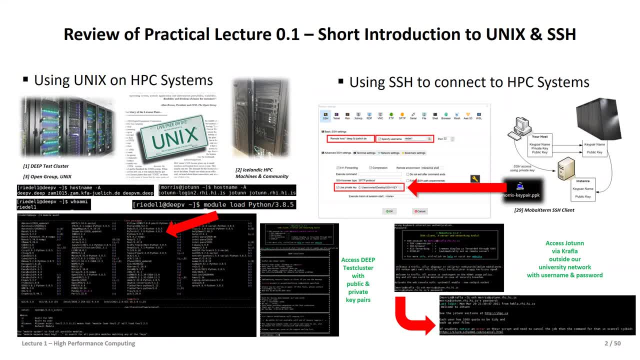 and cannot log in for a while because you have three times did it wrongly. Now we also did this. We also discussed in the course this U-tune cluster And of course this is a very complete, different story. Here we talk about a machine that is purely for teaching. 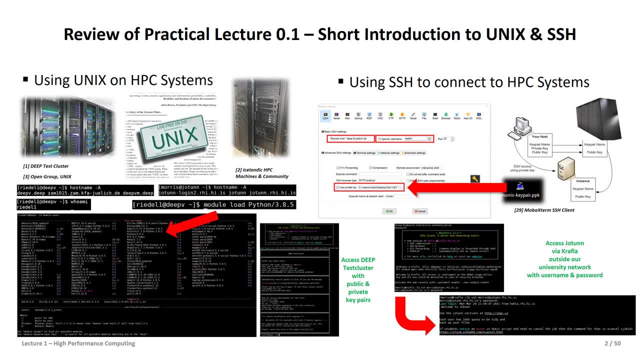 While deepest and deep systems are really for testing in the science and engineering community by real users, U-tune is more or less just a teaching cluster, So the protection, let's say against takeovers and so on, is relatively basically put at less risk. 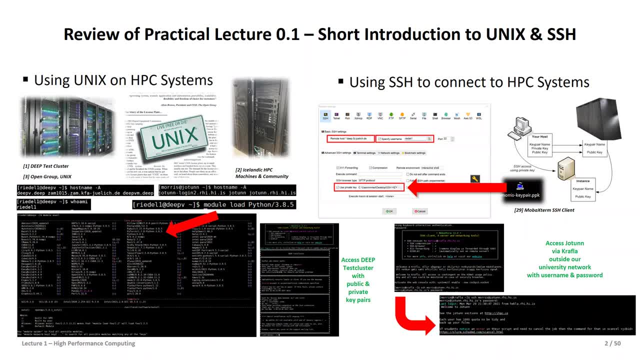 because it's not the most attractive, It's not the most effective system outside, But for us in teaching it's still a very nice cluster where we can play around what we can use to really basically get your initial ideas how to program in parallel. 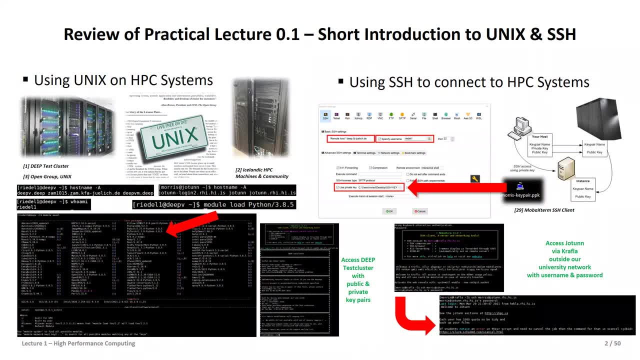 and so on. forward Here we have a system which is protected by username and password, as we learned the last time, but also take away the message that this is in the intranet, So you need to be inside the university network. 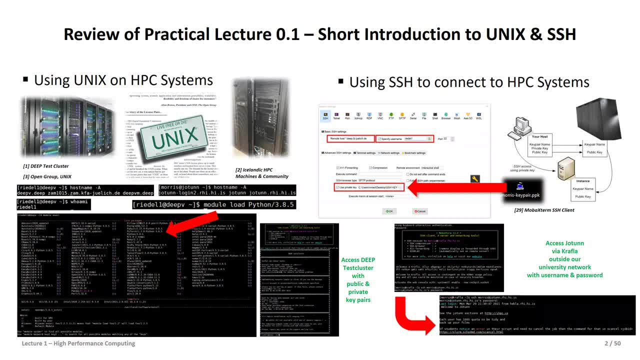 And from there basically can log in. If you're not in the university, like I said, you can log in. You can log in. There's usually a workaround that works, But this also, of course, requires that you can already log in to another system called Krafler. 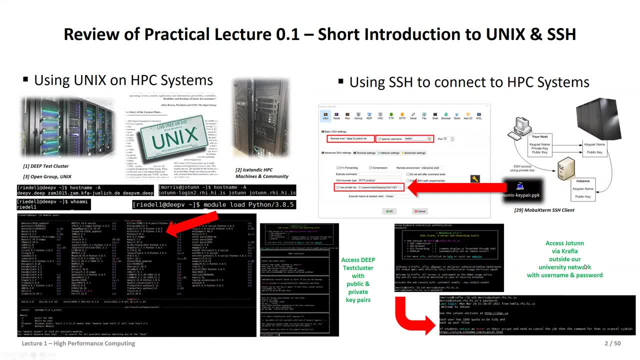 here that we basically discussed the last time, And once you are inside Krafler, you can also within the university network, then make another jump, if you like to, with SSH, as you see here then on the U-tune system. 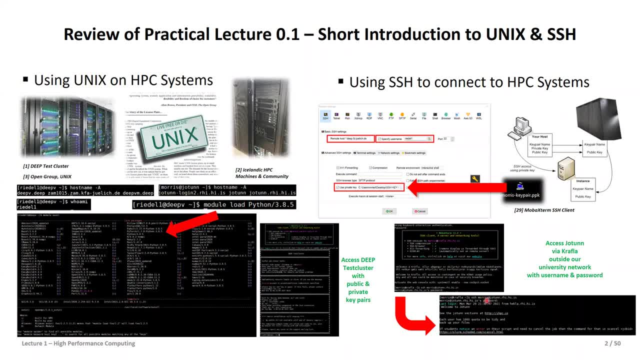 You also realize, with Readle 1 on deep and with Morris here on U-tune, I am completely different identities. I have different usernames on different systems, and that's also usually practice. But let us come now back to the first lecture of the course. 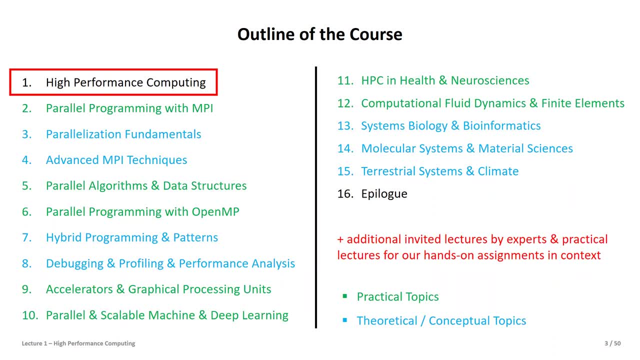 really. the other ones were more or less a bit of warm up and the prologue, of course, a little bit what you can expect from the course and so on, and more administrative topics like what we do in terms of assignments, exams, quizzes. 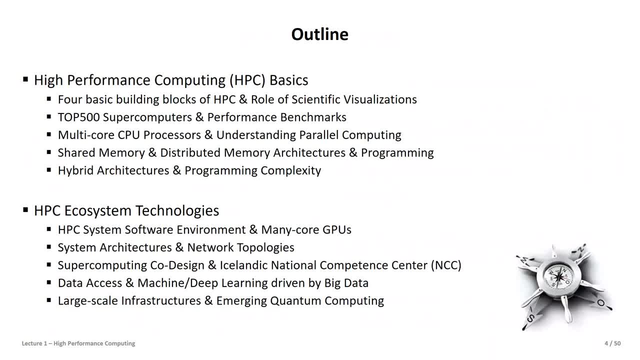 and so on. So high-performance computing is now the first lecture. that brings us some basics. We will discuss a little bit key building blocks of HPC and we cover all of them, of course, in more detail in the subsequent lectures And we'll here and there highlight: 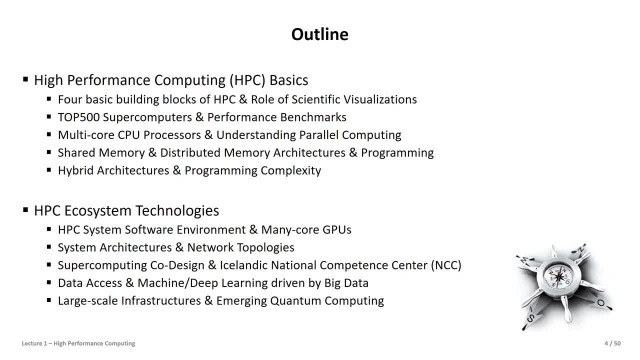 a little bit the role of visualizations along the way. It's a very important list in computing, especially if it's related to supercomputing. This is the top 500 list where we basically have performance benchmarks of the best computers in the world, which then makes them supercomputers. 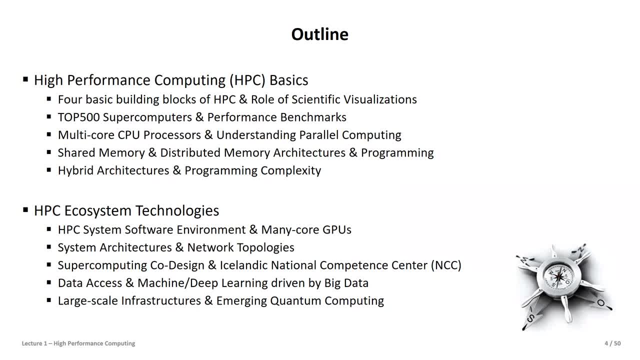 So here we have the term supercomputer that we try to understand, And still we want to understand some key building blocks like the multi-core CPU processor. what is parallel computing? what's the difference between shared memory and distributed memory architectures? and then really how? 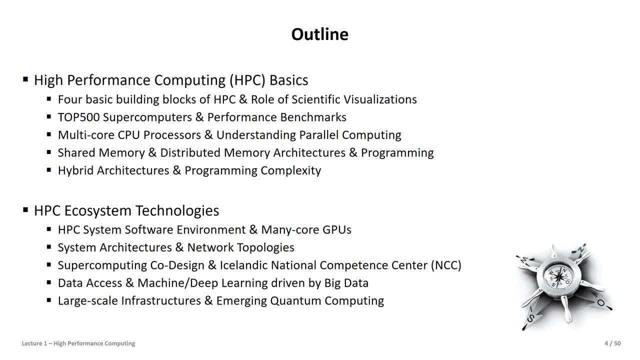 you have this: hybrid architectures that are more or less practiced today and how that relates to some programming complexity. We also will there discuss a little bit the modular supercomputing approach I was alluding to already in the prologue. Then from the ecosystem technologies: 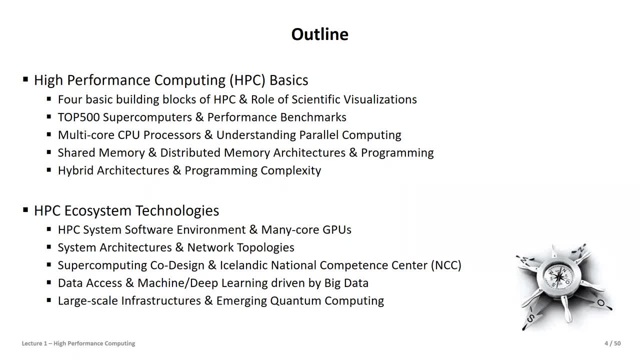 here we're really thinking a little bit about more broader, the software environments. What about the normal CPU and how we go ahead of it? So what could be additions to a normal CPU? We all probably know, And one of those is the GPU, so the graphical processing. 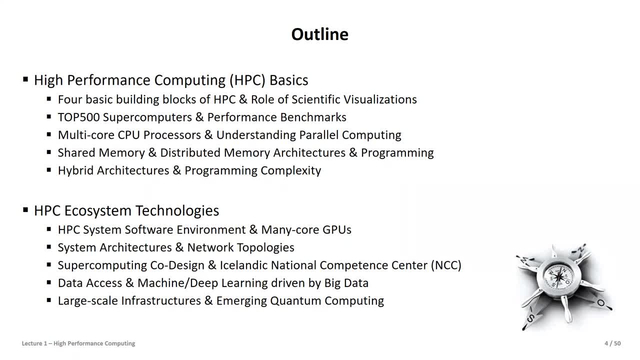 units, which is basically having a high drive these days, for And then of course, we also have a lot of other applications like deep learning, for machine learning applications, but also for many scientific packages and applications, But there are also, of course, many others on the horizon. 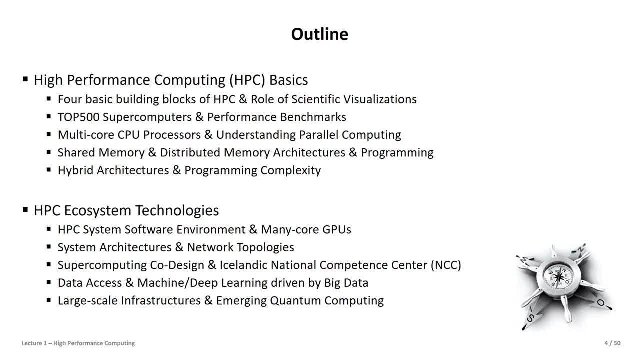 like graph CPUs, like neuromorphic CPUs, and some of you have already heard from quantum. So we will discuss this a little bit in this particular part of this lecture today, And with this I also want to give you a little bit of an overview of what 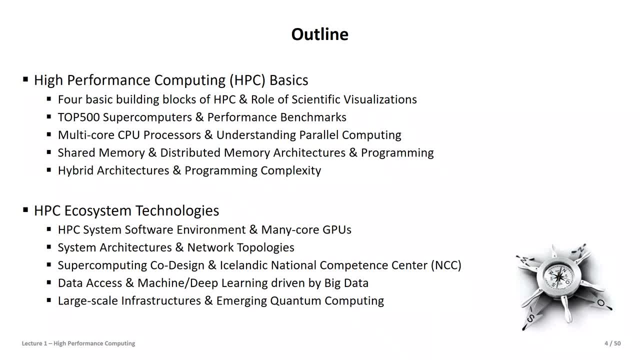 we're talking about in the next few minutes. So we're going to start with the. So where are we? How it relates to the EuroHPC joint undertaking, which is also very important now in the light of the new course here Since a long time, and elements of those. 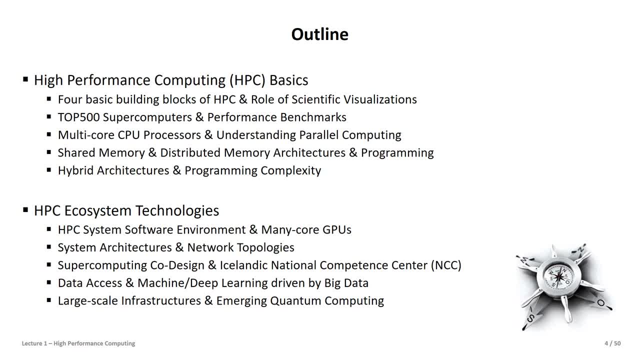 are now transitioning towards EuroHPC and we will talk about it. And I end the lecture a little bit with a small hint of what we do already in quantum computing. It's not future. We have already several publications. We have a physical system in Jülich, for example. 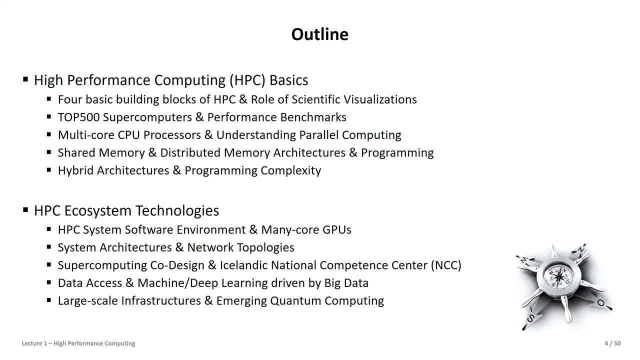 which will be inaugurated actually next week, And with this we all basically can see that quantum computing is not really the future In the long, long, long distant future. it is there today And this is also an important example of HPC. 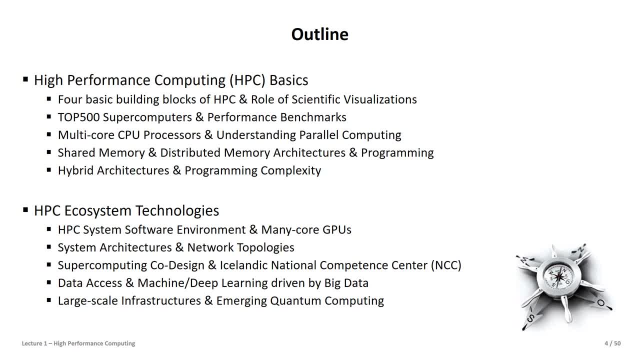 New technologies come around, like GPUs 10 years ago or maybe 15 years ago, and suddenly they are there. We deal with them- new programming paradigms, And this is also what HPC makes it so interesting. So let us start with thinking about the learning outcomes. 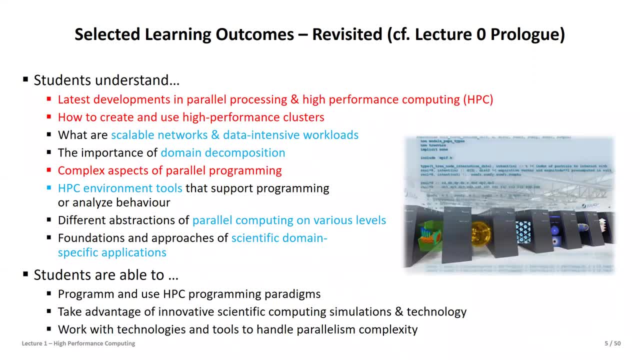 here We deal a little bit with the latest developments, really in parallel processing and HPC And of course on a reasonable, let's say moderate, level. still we will not go in deep MPI programming, But still you will understand the complexity. 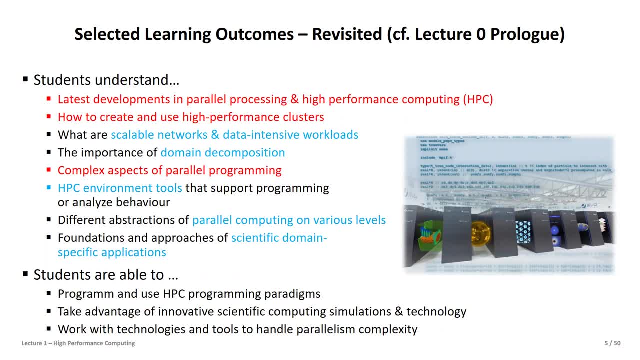 of parallel programming. What means when I cannot access a memory which is usually very important for computing? So when you can't do that, how you deal with it? You have, let's say, message passing, You have distributed memory, But how that all works was in the kind of architecture. 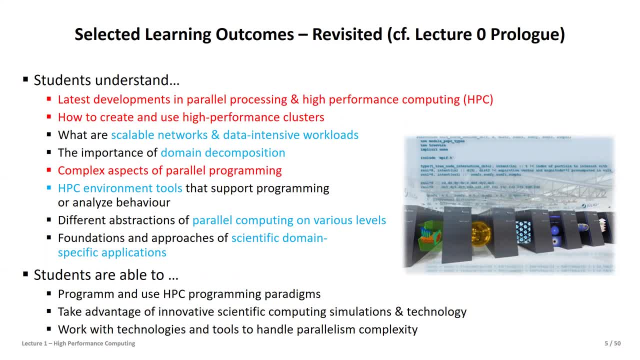 that then creates this HPC machine, And with that we will talk about the future, And with this we are basically also able to think about how we can create and use those HPC clusters. really, because you will also realize, it's part of this lecture. 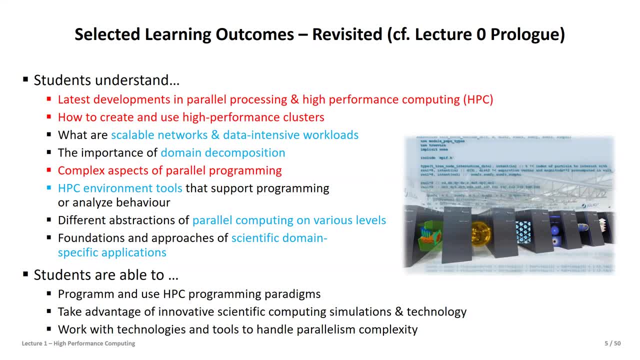 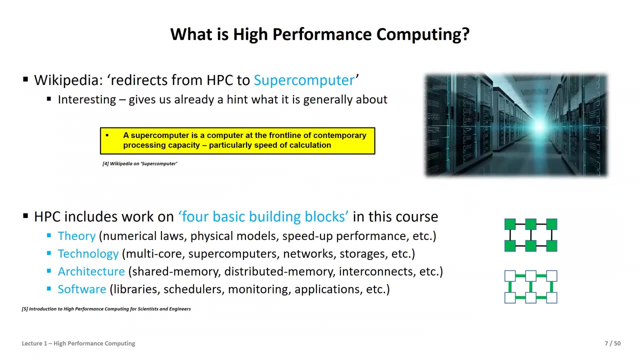 They are all basically based on smaller parts like recs, note cards and so on, And this brings a lot of chips together. So let's start with the real part, one where we try to reveal a little bit what a supercomputer is. 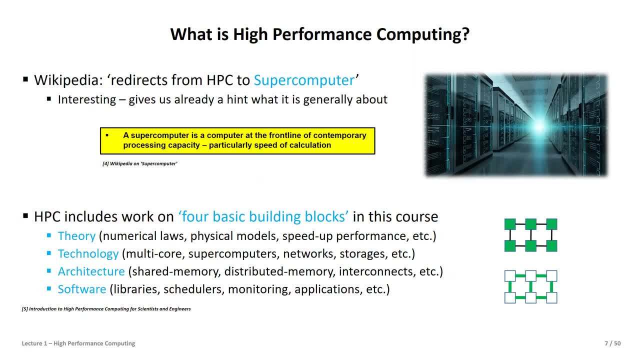 And it's a loaded term, perhaps A supercomputer, And here's a definition. if you want from Wikipedia, You'll find many others. There's perhaps not the one and only definition around it, But they all share the common view of that. it's really. 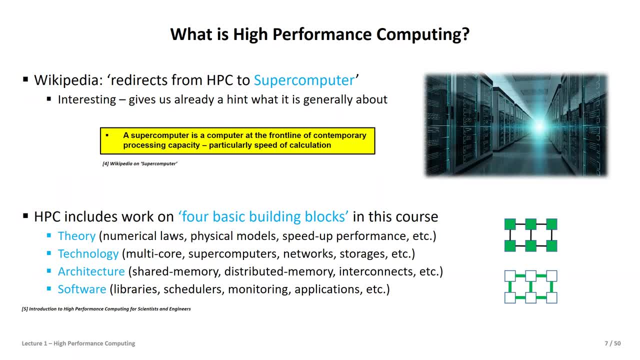 the Formula One of computing. So here you talk about computers really being at the front line of the processing capacity, capability, And with this we can solve problems we never can solve before. Or we basically can solve problems with a much more granularity, with much, much more. 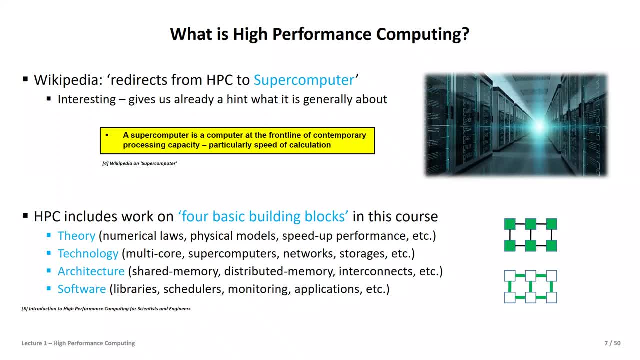 complexity, With much more understanding, with much more precision. There are lots of good examples why it is a supercomputer And when you talk about the course topics, in a way you can categorize them in these four building blocks, which I would say is roughly what HPC stands for. 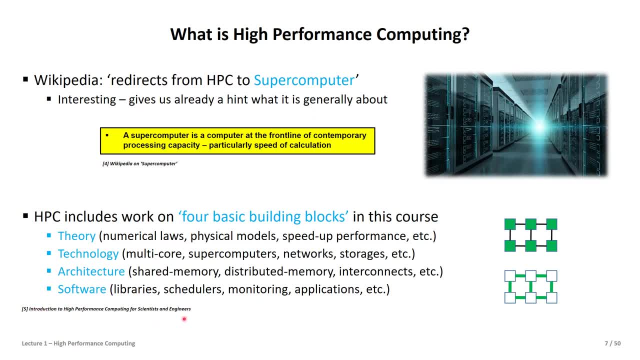 And if you want to read more about this, there's also this book I mentioned in the prologue Here, the Introduction to High Performance Computing for Scientists and Engineers. It's a quite interesting book for these basic building blocks, But still, when we go, 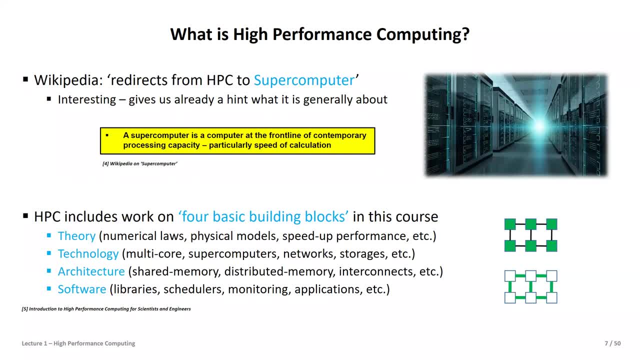 For other topics we go more for references online or in the community. So we would see that HPC includes theory, a lot of theory. So physical models, which are the applications we run on the systems. We want to understand the speedup in some of the lectures. 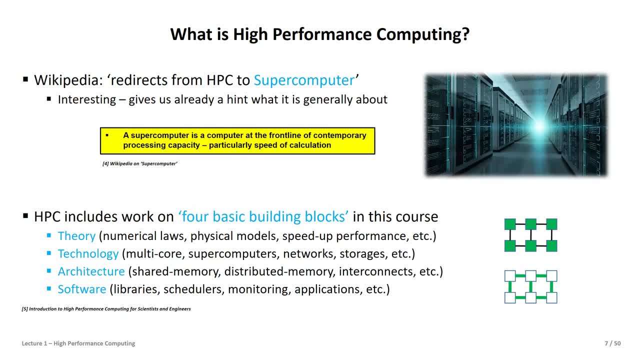 which is really the idea of saying high performance. So we have to measure performance to understand the speedup. Does it really use or is it useful to really basically combine different CPUs to tackle a problem? So this is what we want to analyze. 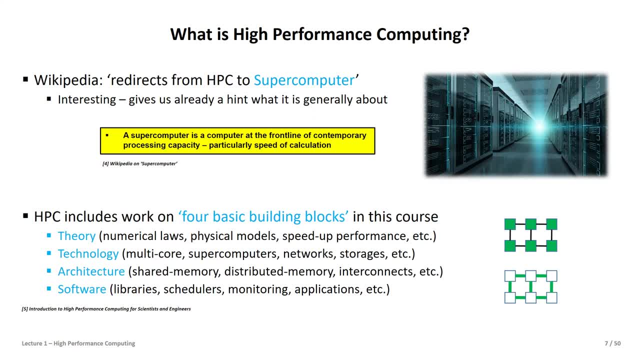 We do performance analysis to understand problems, bottlenecks, and that makes it also HPC. There's lots of technologies out there And the whole of the course you will see was many cores, multi-cores. We have different network topologies. 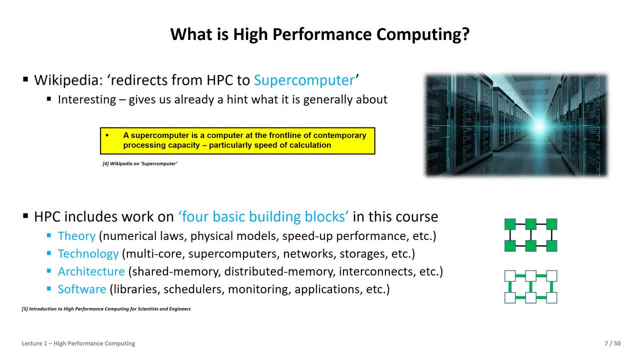 Dragonfly- basically relatively new now when you compare it to maybe 15 years ago. Again, storages, the storage hierarchies, caches, So this will be all Parts Of the course. Every now and then we will review this. 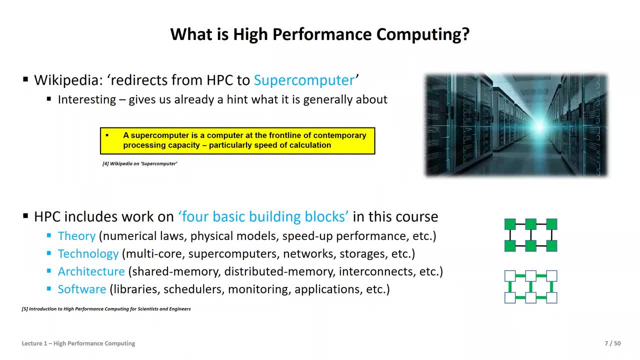 And this lecture starts a little bit with the technology, blueprints of shared memory, distributed memory, which makes it certain different architectures, Because you can combine these technologies, of course, in different ways, You can have different interconnects. The interconnect here in HPC is very important. 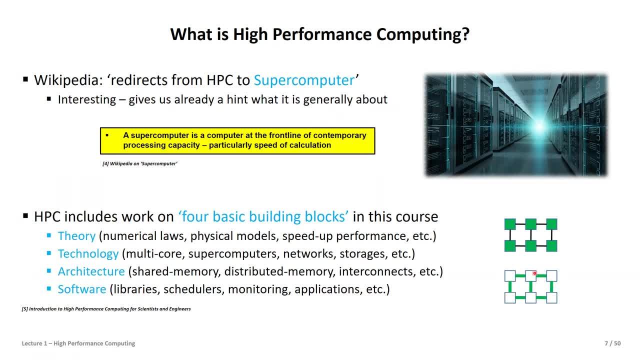 Basically you see that a little bit explored here in this kind of figure where computing is a very important part in HPC, No doubt, But of course the interconnection between those different nodes and so on is a very important part with high interconnects. 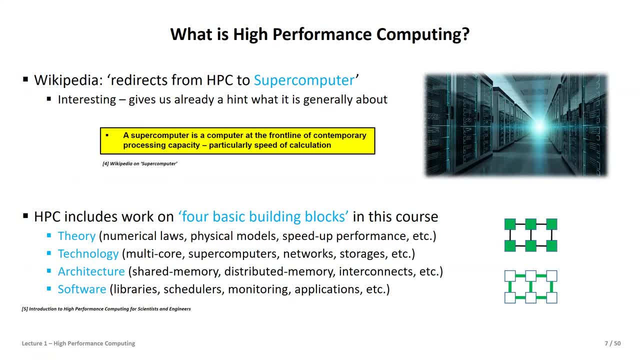 like Mellanox provides, for instance. And then there's software libraries, applications, but also administrative tools like monitoring and schedulers and so on, And this is also one of the ideas I will provide to you actually tomorrow, when we talk about essentially 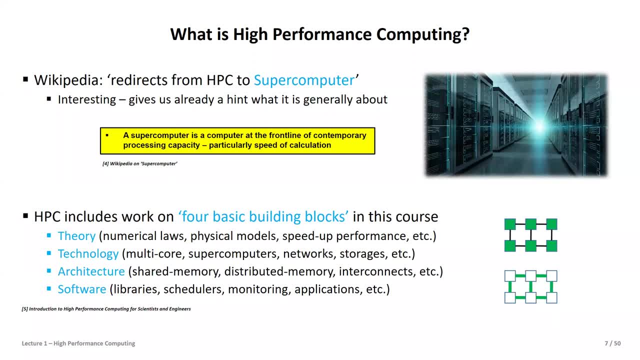 than the other practical lecture, one one. so the next lecture will be really again a practical lecture where you show a little bit what means really scheduling. so this will be more practically then, but very important for hpc, meaning that there are lots of different users on one system. 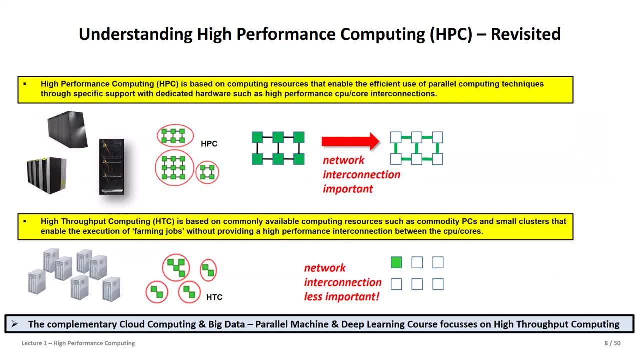 at the same time. so again, when we think about the high performance computing term, these are definitions which are more or less principles. really in computing you would say high performance compute is really computing but has a very high in performance interconnect between all of those different cores, no matter how many of those are existing. the interconnect is very well. so you can. 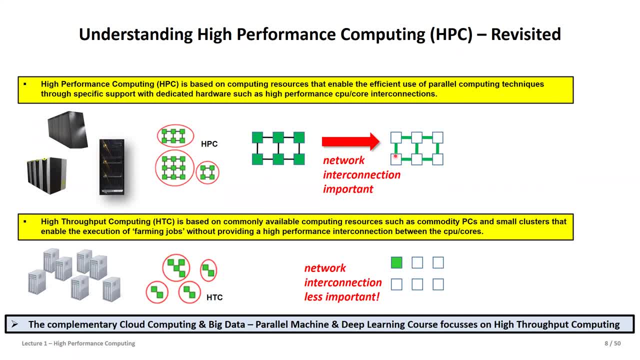 use them brilliantly in parallel um, basically with low latencies to it, and can enable certain applications where your neighbor or getting the connections and the communication to the neighbor is incredibly important, like weather forecast for some, for example. now, another term which stands the test of time is high throughput computing and 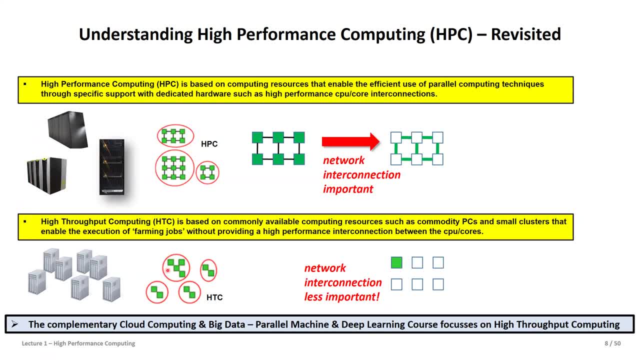 this is usually where we basically contrast hpc a little bit. we would say there are lots of computing maybe in different cores, but usually they're not so much well interconnected. they maybe just use ethernet and you come to a situation where the network connection is maybe also not so important. 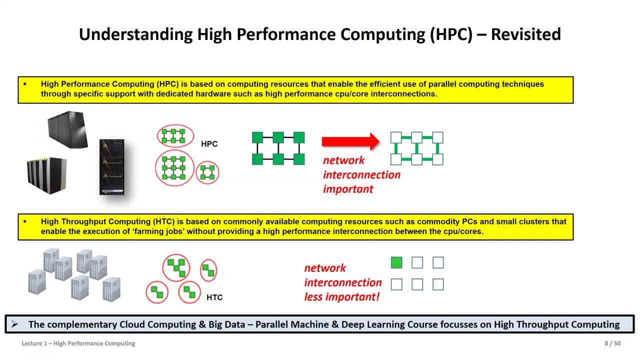 an idea is, maybe, if you look through many documents- let's say 20 million documents- in terms of a network provider or a news provider, if you want, a news provider might be a good example, where you have, let's say, different topics about politics, sports, and if you want to basically do some statistics on this, 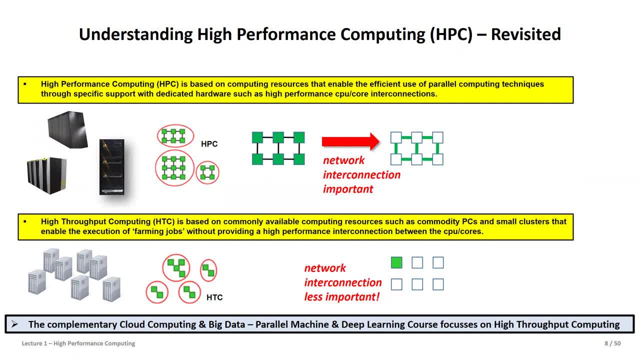 how many basically have been in sports? how many have been on politics? how many news articles have been run? you just can do this by breaking up the big problem into smaller chunks of a couple of millions and putting them to the different computing entities in between. they don't. 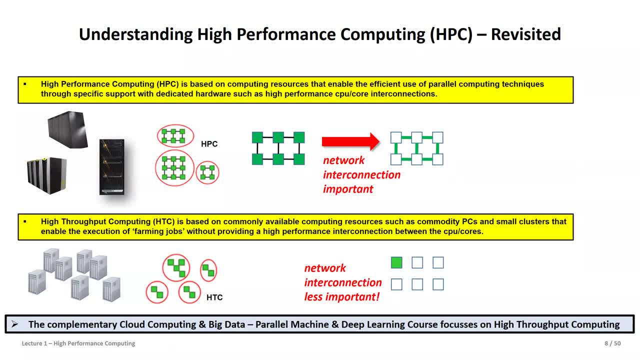 have to interact. they don't have to talk to each other. they can solve the problem more or less independently, parallel, or nicely parallel, as someone in our community would say. so the interconnect is not so important. you maybe want to have summary statistics, of course, in the end. 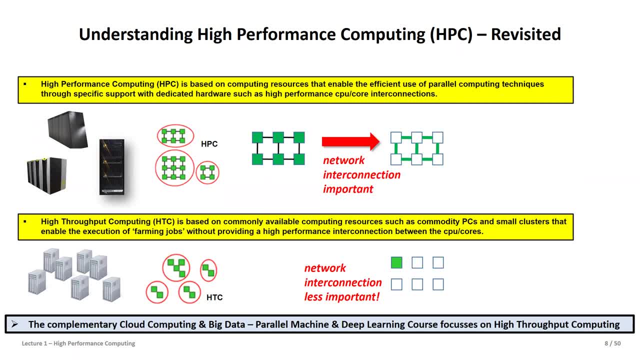 you want to have the big picture, but this doesn't require on every little second to interconnect or basically to communicate than really with your neighbor. And this is, of course, a complete difference if you think you would use these six here for weather forecasts, and they want to basically predict the weather. 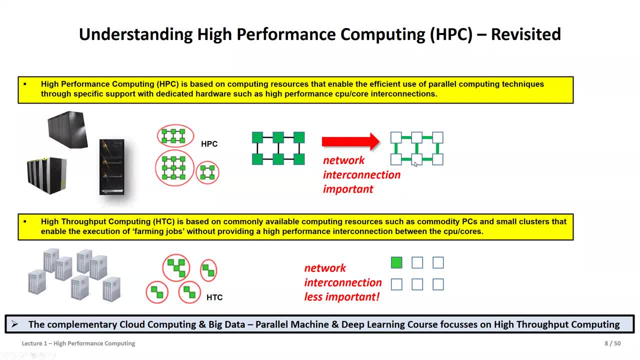 and in order to compute the weather every little second, you need information from your neighboring CPUs or cores or whatever it is you parallelize on And with this these two different principles stand, and it's very important to know by heart. I also give a short indicator. 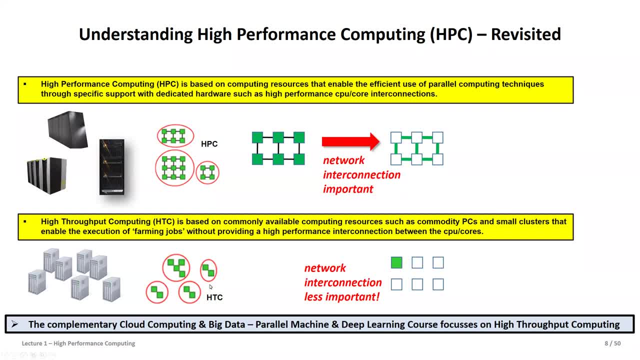 that in our complimentary cloud computing big data course we focus here and there much more in the HTC paradigm, which is also much more often in clouds, Although some HPC machines, of course, are also part of basically clouds today, Now when it means parallel computing. 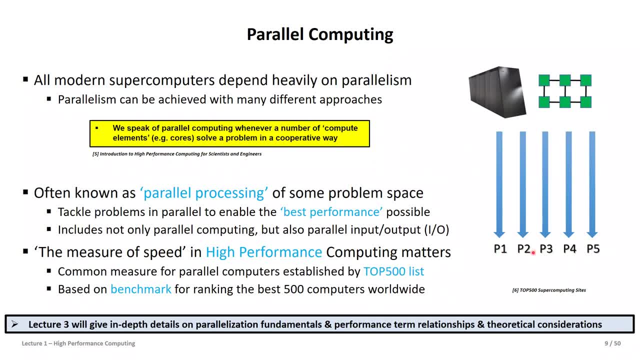 we usually say that all these different processors basically solve some form of a problem, of a scientific challenge, of an engineering construction simulation, but in a kind of cooperative way They work all together to solve that problem And it's known as power processing and so on. 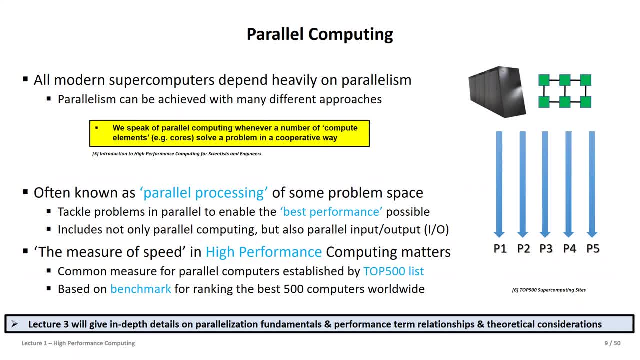 but here it's very important also to think about that. this, of course, not only means pure computing. If you have real engineering problems or scientific application, you will see that data- so parallel IO input output- also plays into the game. Now, of course, we want to do this with high performance. 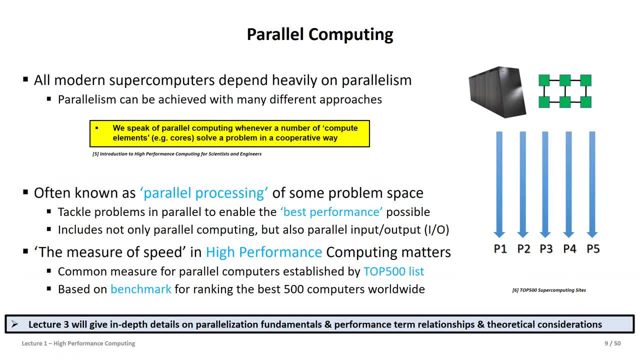 but before we do this we also want to understand what high performance really means. and you see, here in lecture three we will go into much more details what this parallelization really entails and give you also some performance relationships and theory. but let us look a little bit. 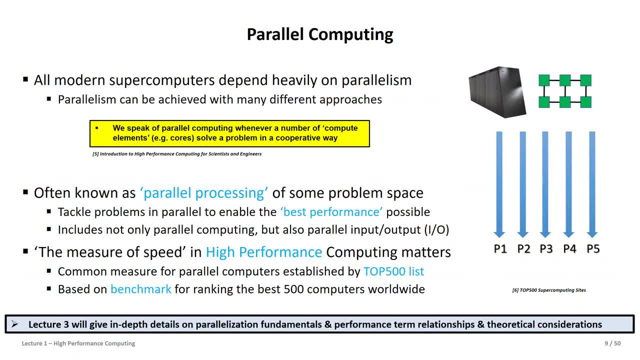 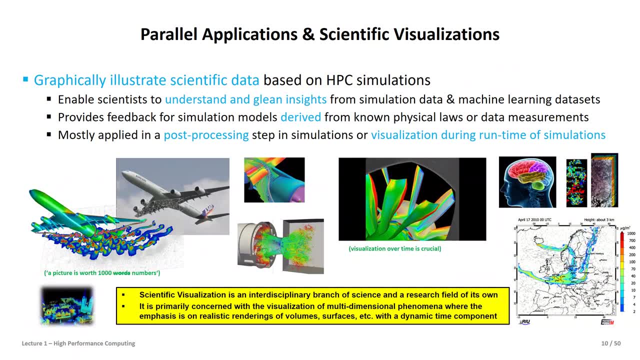 what this top 500 list now is, how it is actually based and why is that existing? So, essentially, you think that you know, parallelizing a problem could be always equal. So just throwing two cores or three cores at it, it will be, of course, double as fast, or three times, you know. 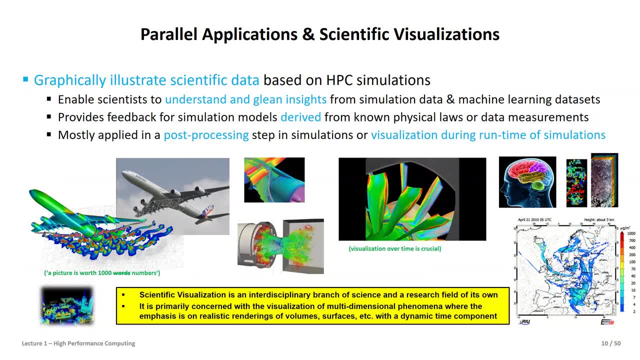 it will be, of course, double as fast or three times, you know. it will be, of course, double as fast or three times, you know, as fast as using just one core. But the interesting thing is that in HPC, many of these systems really are running. 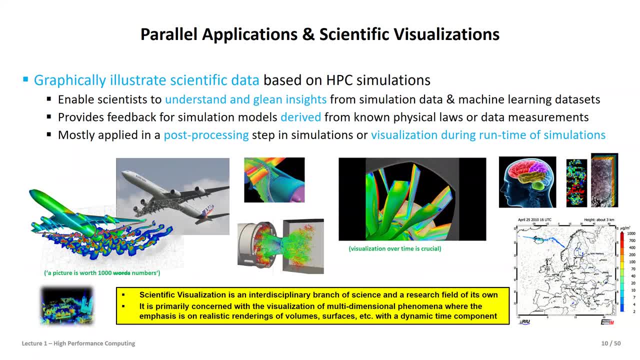 a lot of applications where the performance as such is of course also very application specific. So here you see several parallel applications that really also drive the demand for HPC systems, An Airbus, for instance, that you have here. basically that is, you know. 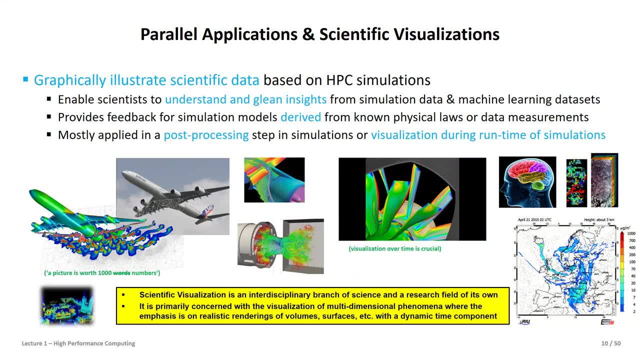 modeled via so-called computational fluid dynamics simulation point cloud examples building the buildings back with basically clustering algorithms and HPC and all the engineering parts here And you have a simulation over time which is mostly interesting, like this wheel: here you see basically the turbine here of an aircraft. 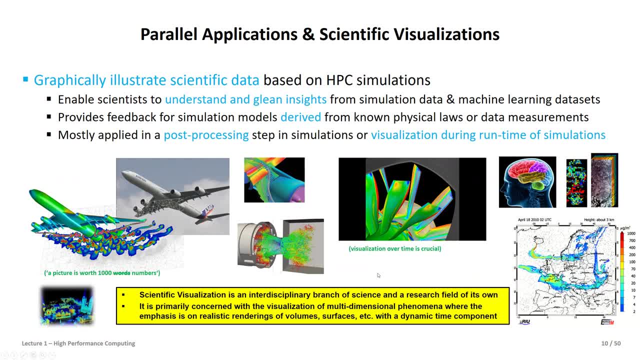 And there are lots of these visualization that really are a helpful tool to understand what's happening in these scientific simulations, And this is valid for brain sciences, for remote sensing, So using satellite images and then essentially spectral channels of light here, which makes it a cube for analysis in AI. 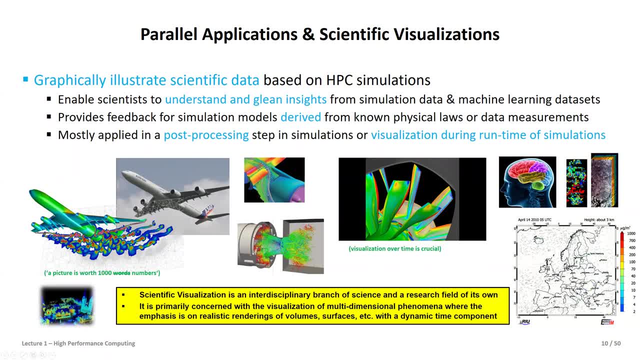 which we will also talk about when we talk about deep learning. You see here the Ia, Fethi Ayurkul, where the particles really run over Europe and shut down the air traffic. So the visualization are really helpful and, in a way, are always alongside the HPC. 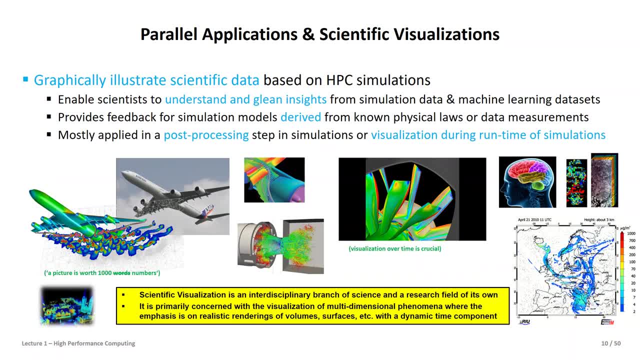 And this is because basically the simulations are usually very complex and multidimensional problems or phenomena which really then helps to visualize, so that basically people can understand it much better than just looking on multidimensional arrays which are sort of very cold, but here you really in an instant can understand the situation. 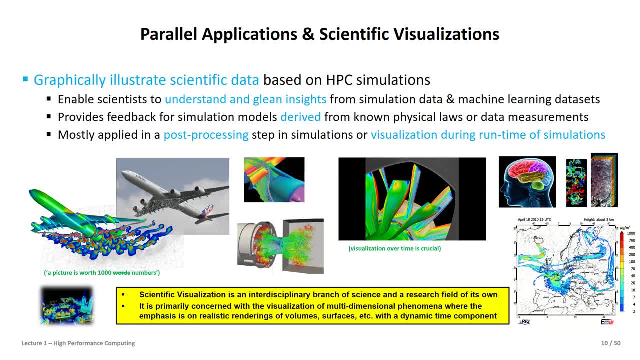 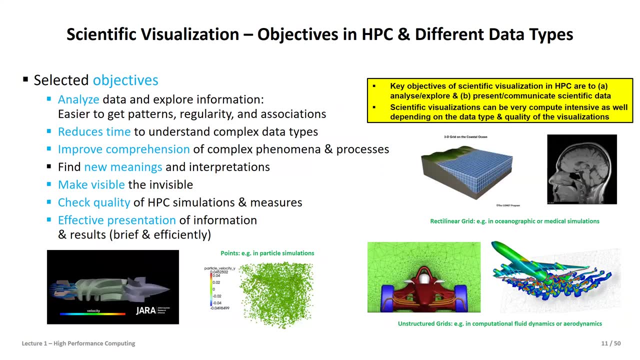 of this cloud, for instance, of the ashes that we have seen over Europe affecting the flights, and of course, the same is true for the pictures here from the aircraft brain and so on. so scientific visualization is very important. it's really reducing the time to understand these complex setups. it also makes us understand that we often break the big problem in smaller chunks. 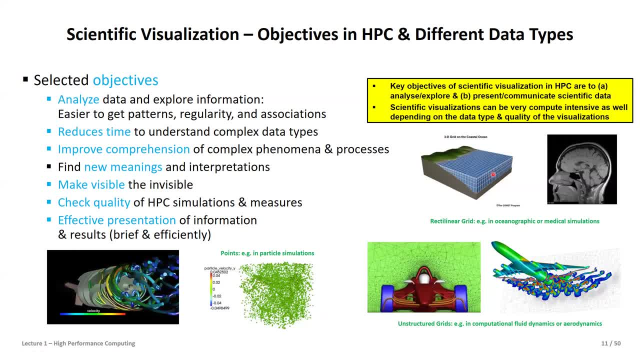 you see here a very homogeneous cut of a 3d grid in the coastal area. maybe you want to understand a little bit. you know what's happening here in one of the interesting fjords or so in Iceland, so you would model that maybe more homogeneously in. 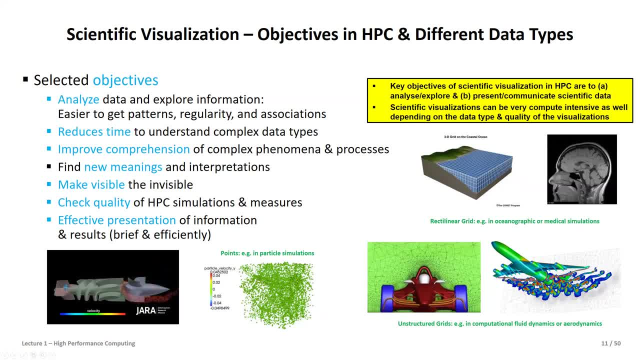 the beginning. once you have then really, let's say, several structures, you would say you would go to a fine-grained mesh and you see here the formula one car where lots of computing is happening around with the airflow around that. where the mesh is relatively small, you have other. 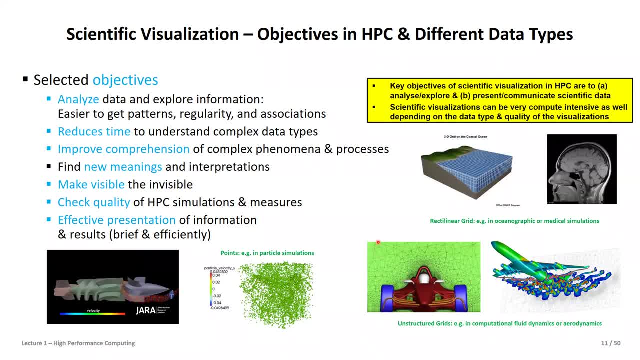 areas where the formula one car is not affecting very much, where the mesh is relatively coarse grained, and of course the same is true for the aircraft brain and so on and so forth. so you'd have an idea of what's going on in the third and fourth dimension for an aircraft wing in fluid. 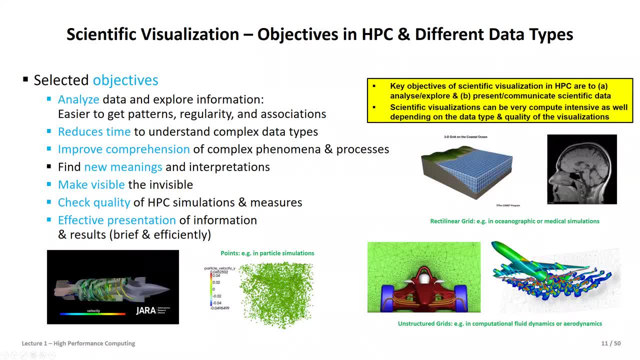 dynamics, but of course you can think about also that this will be a topic we will talk about later on much more in detail so that you can better understand it. or here you have also the blood pump that shows you basically the velocity of the accelerated blood which should be inside. 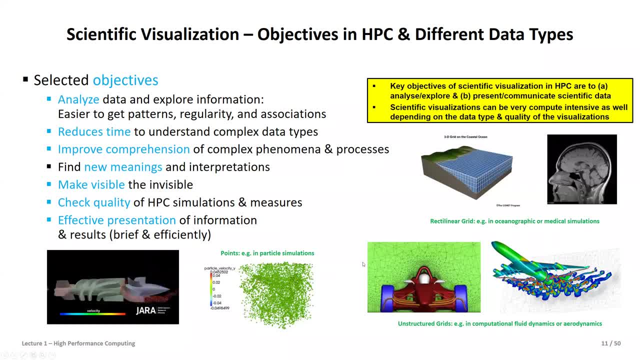 the body. so no matter where you go- in medicine, in earth sciences, in engineering sciences- it is invisible, as we say, and really helps us. the understanding also, when you come to the world of the small or the very small in particle simulations here, what is the density, what is? 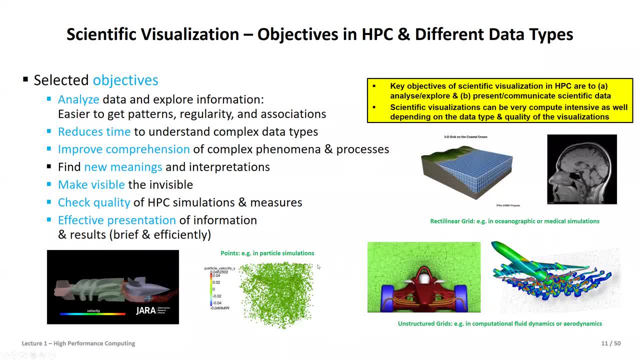 the velocity of the particles. it's all something we talk about, but it's important to understand that this is usually a very important part of hpc: to analyze it, to explore it, but also then to communicate- maybe to decision makers and to basically other users, what we will do with data. 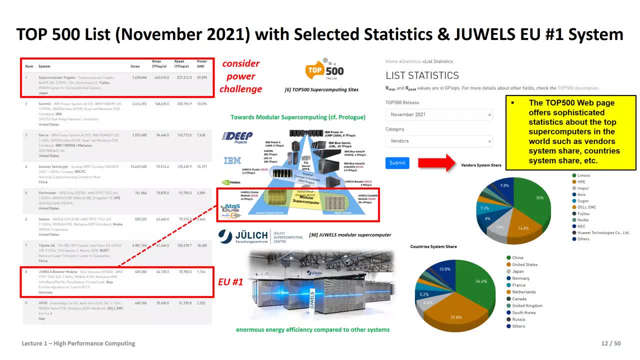 what is basically the simulation about now coming back that these applications are now really driving the demand for high performance computing, but we still not really clarified what that really is. so who says it's high performance and what are supercomputers? so there's one specific list. 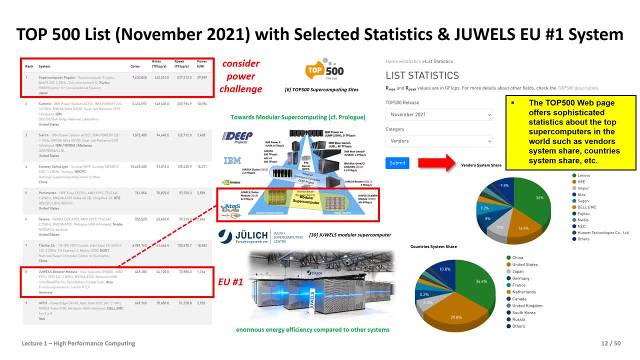 in the world that nails it or anchor it a little bit. of course, you would say that this list is, let's say, a bit, uh, controversial. It just, you know, measures in a certain benchmark, the best computing. But, as I said earlier, the different applications have their different requirements. memory computing accelerators. 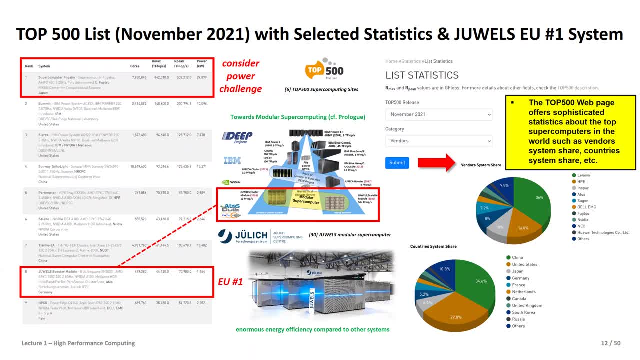 So probably it's not that easy to say it's the most important system. You rather would say what is the most important system for this and that application And for this also, the top 500 list has created more lists now, So we have a green 500 list being more for the efficient energy efficiency. 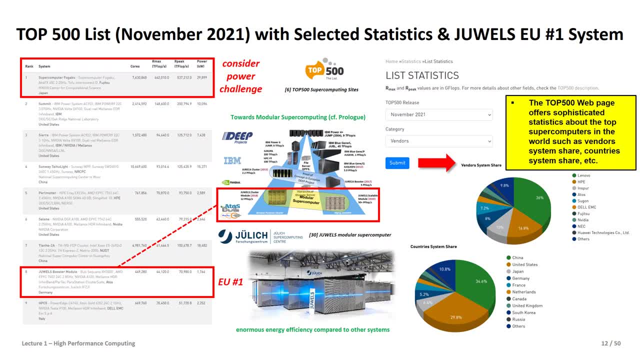 We have the graph 500 list for more graph problems to solve, And here's the top 500 list, which is of course the most famous one, where you see essentially the best computer in the world with 7 million cores. Very interesting, a very specific interconnect. 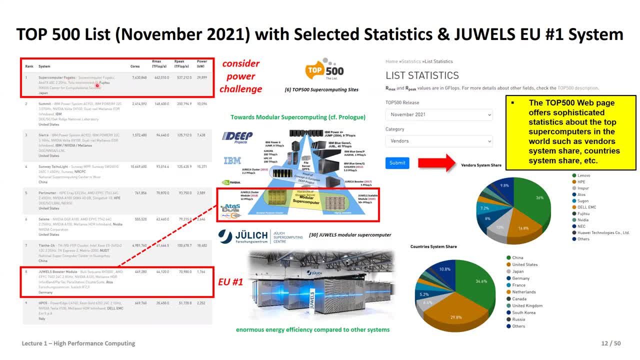 As I said, HPC is defined by a very good interconnect, While here Tofu interconnect is a very specific one from Japan. We, for instance, here in Jülich- having number one in Europe and number eight in the world- currently have the InfiniBand and Mellanox interconnect, which basically enables us also to use high performance. 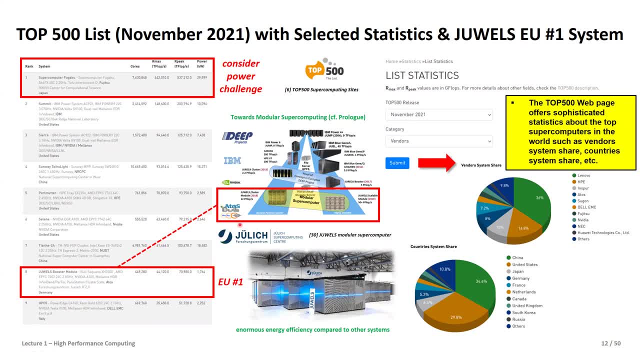 And in between is a lot of space And particularly I want to highlight the power challenge here. So you see the kilowatts here where basically Japan number one, obviously with 7 million cores, requires lots of energy But is also a big footprint. 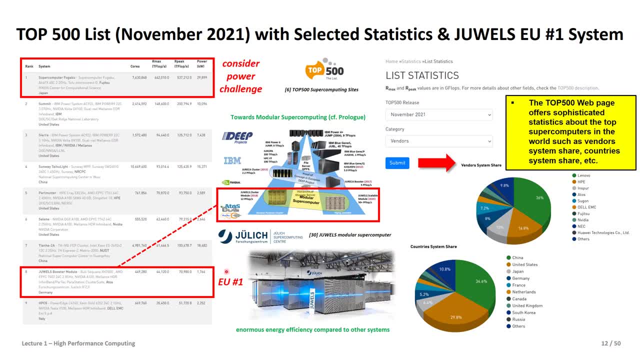 In money and also, of course, in our responsibility to nature. And when you see that number 80 in Jülich compared to the predecessors here is a very high performance system, being very energy efficient and having a fraction of the cores and basically a modular system architecture, as we already discussed before in our prologue lecture. 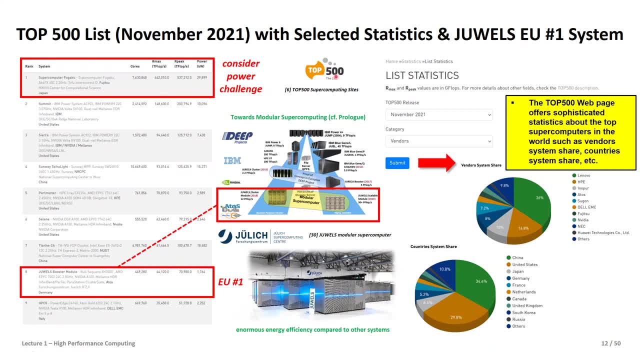 Just for you to explore. I would encourage you to go to the top 500 list Because it's a very interactive list. It's not so cold as it is shown here. Obviously, Europe has a part to play, But we see that in the last years, or maybe the decades- I'm now 18 years in Jülich. 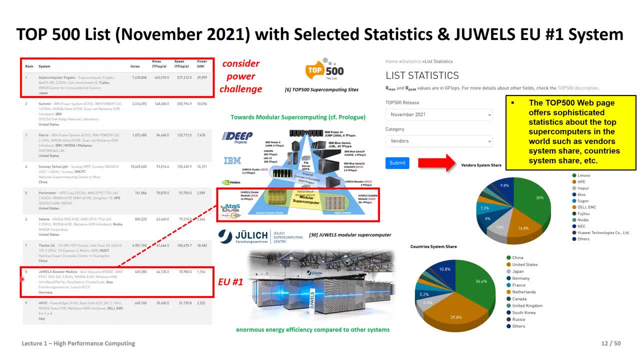 We have been once number two or so in the world. We in Europe actually fall more down these days And we see China and US, of course, being, together with Japan, always basically the leading drive these days in terms of the top 500.. 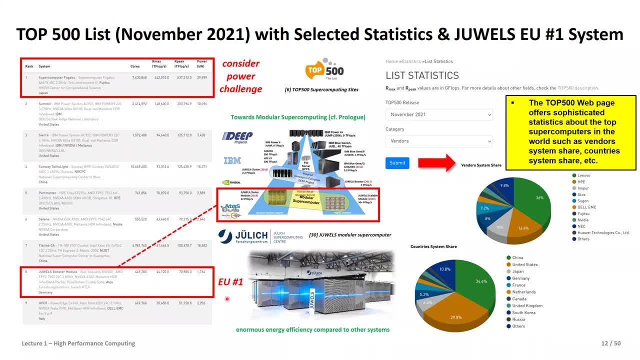 But you see, also Italy is coming again into the list and some European countries make it also to very large systems. But this is of course something you can explore much more interestingly interactively, when you go to the list statistics, for instance. 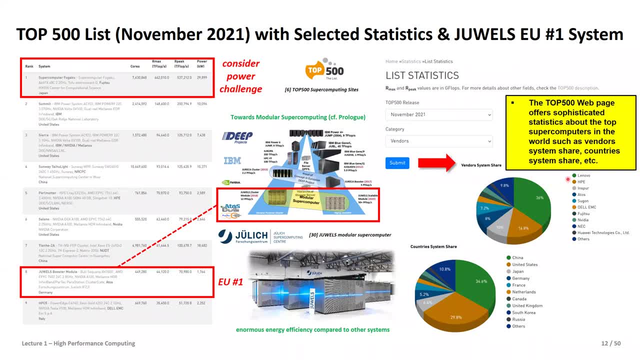 you have things like vendors share. that might be quite interesting. EBM transformed to Lenovo, So still essentially the legacy of EBM, so to speak, is still in the game. You have HPE, which is more or less some parts of Cray, which 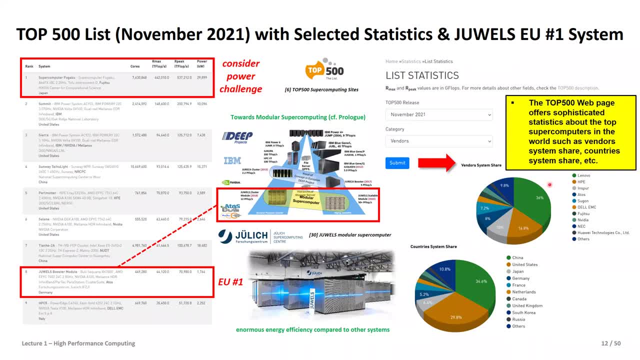 you know, some of you probably never heard as students, But Cray was a very long player in the HPC community So and we have new players, like Atos being, of course, very important in Europe, playing there, a key part of infrastructure and maybe basically a vendor of HPC in the. 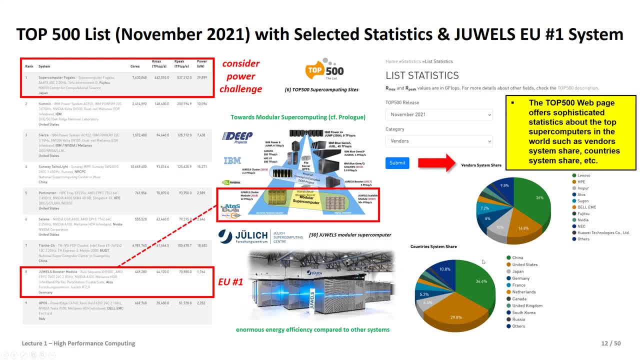 future and architecture and so on. for the countries, I have to say we see that China, United States and Japan really make a big place. The numbers change here and there, And last year China was a bit more into the list And now the United States actually pick up a little bit. 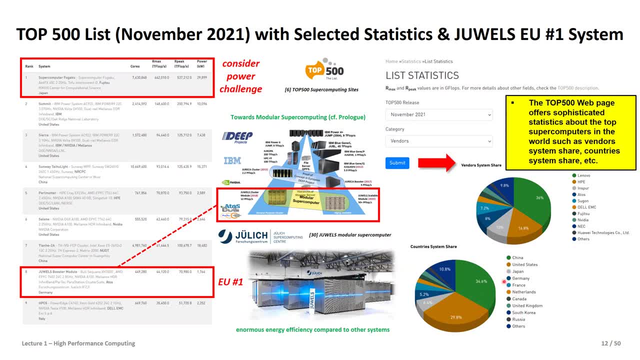 And we see that some European countries are still in the game. But it's really defined by US and Asia, largely saying China and Japan these days. So Germany, as you see, is still a big player too. Over the years we could in Jülich at least sustain, and also more broadly. 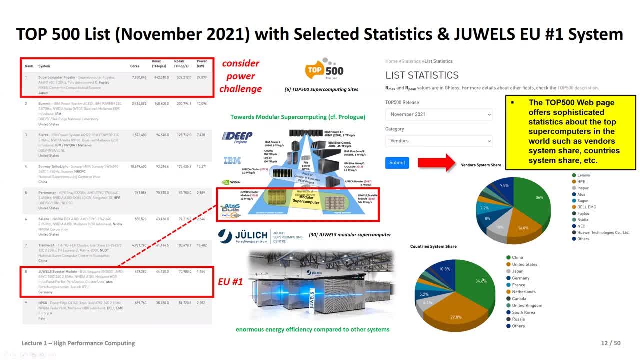 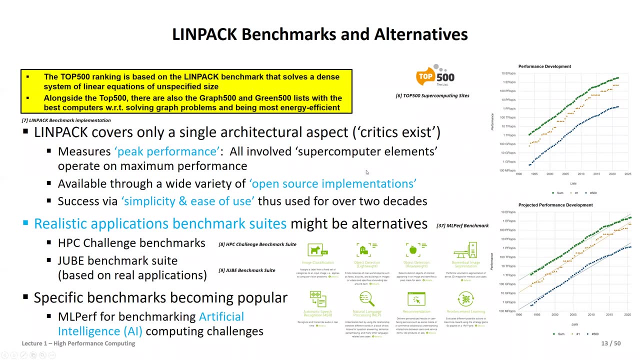 speaking with the Gauss Center for Computing in Germany, sustain also their high presence, but still basically something in orders of magnitudes, as you see from the percentage. So explore the list. You will see other statistics. You will see details about the top 500. 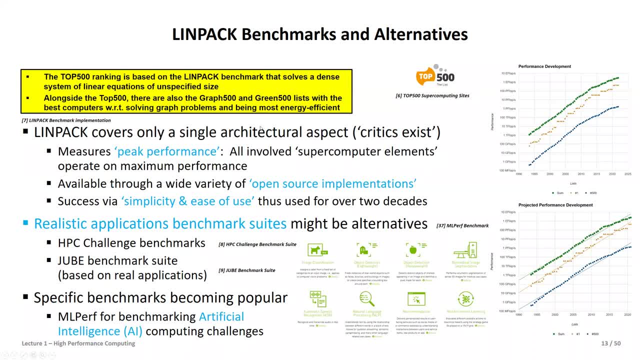 So LINPACK is a benchmark which is used solving a dense system of linear equations of an unspecified size. But with this also comes critics, because most of those should be having much more realistic application benchmarks these days, and that's why everybody says in the community top 500 is important. 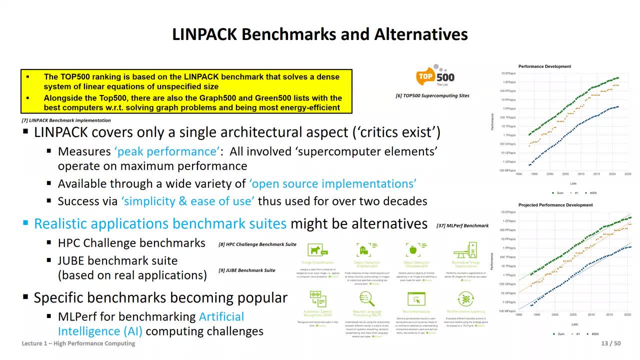 for, to see the general computing capacity, the capability. But when it comes to real applications, you know this is not really the statement. You have to really go with application specific benchmarks to understand and really know if the system is really good for a certain application. 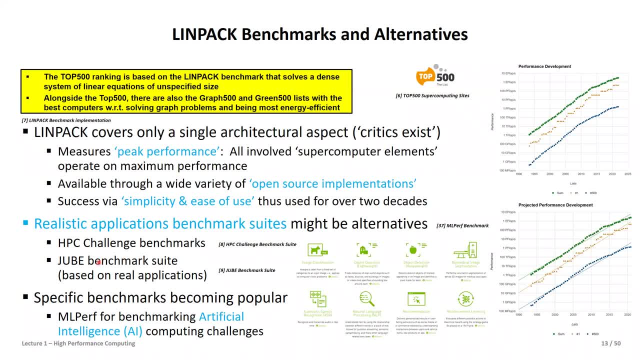 So they are challenge benchmarks. These days, there's a huge benchmarks for smaller real applications And we see more specific ones, like MLPerf, for instance, gaining attraction in the community of HPC, in particular, in the context of artificial intelligence. 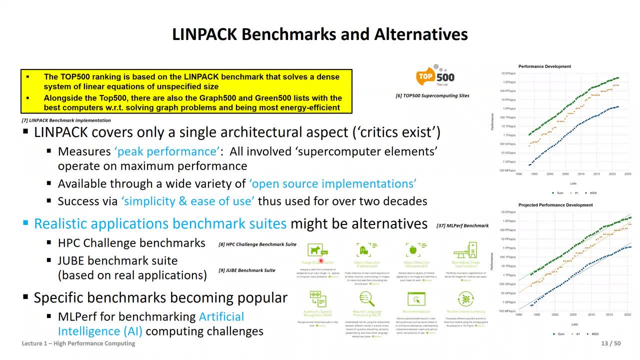 where you see here some basically parts of it: image classification, natural language processing, challenges. So this is another very specific benchmark where HPC is judged on. An interesting part also is one of the statistics in the list Where you see on the upper part here, of course. 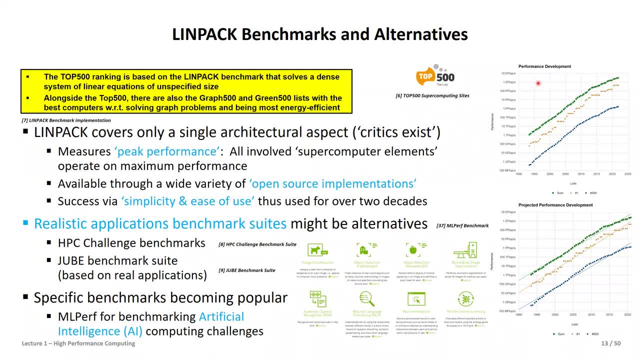 is the sum of all these computing capacities which now reached exascale. And you know, in the product we discussed a little bit, this 10 to the 15,, 10 to the 18, where we're going to now, And you see the lower part of the top 500, but also the upper part. 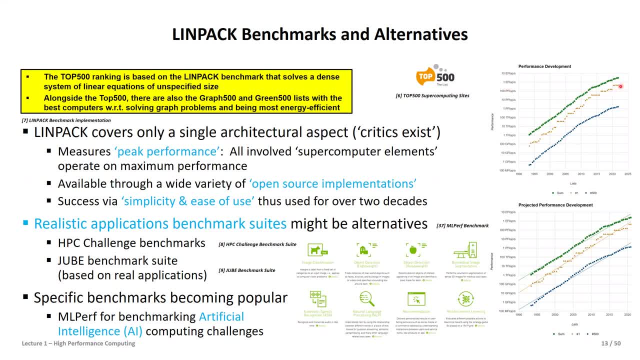 meaning that we almost are there of having exascale systems. So almost is a loaded term because exascale systems Are quite a big endeavor and very costly. But the chances are that essentially in the next two years- 2023,, 2024,. 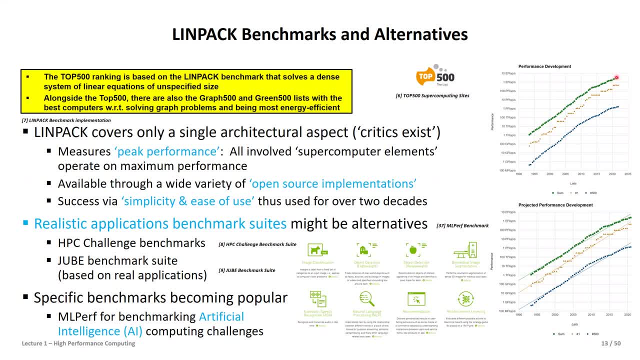 we probably see the first exascale system stand alone and then of course also driving higher the summary of all the computing power in the list. Also here. this means in the development, the directions you could see more or less. it is still growing constantly over the years. 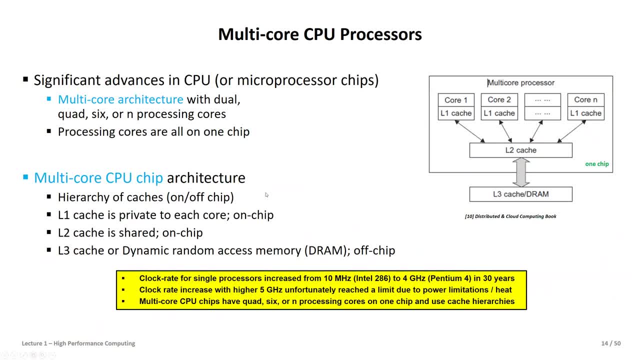 And there's also something we can expect in the future. Now a little bit to the architecture elements, and actually some of you that have taken the cloud computing big data course, of course, have seen these basic parts as well. So we have now CPUs and there are some ever. 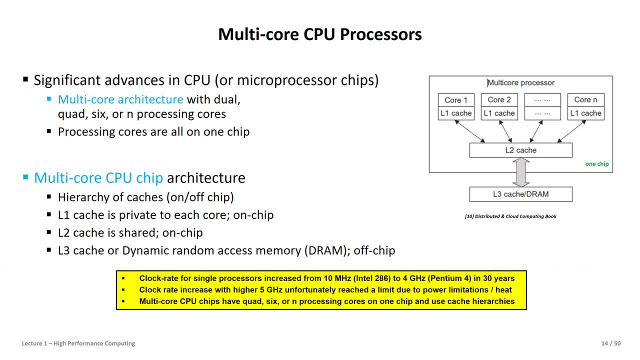 increasing amount of, you know, power in the CPU, meaning there are caches, different level of caches, and you have, let's say, many more cores on it, But still it's limited. It's not thousands, of course. 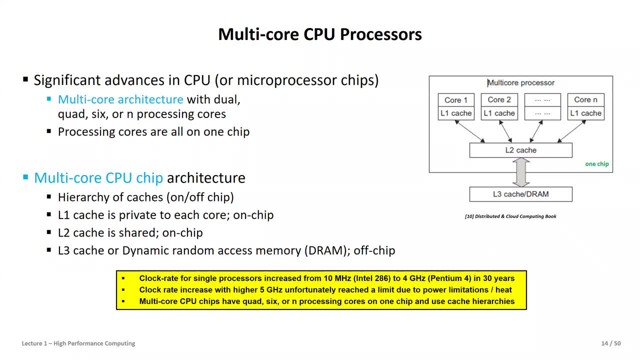 Here we're talking about the multi-core chip that has single-thread or high single-thread performance, And the problem is here that these chips are getting too hot and you basically end up with a problem that there will be too many errors in the chip, So you cannot advance there forever, creating more and more better chips. 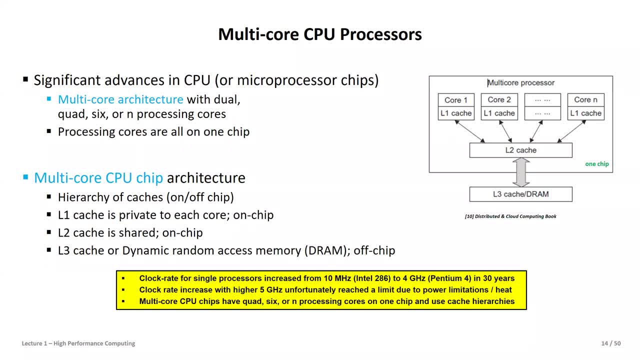 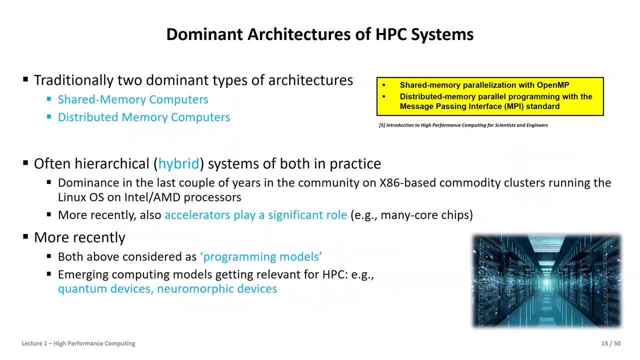 And, as such, many core GPUs are now existing where the cores basically are not that powerful anymore. but you can put thousands on the chip. Still, of course, the systems that we have in the HPC systems are very powerful. We use cutting-edge CPUs. 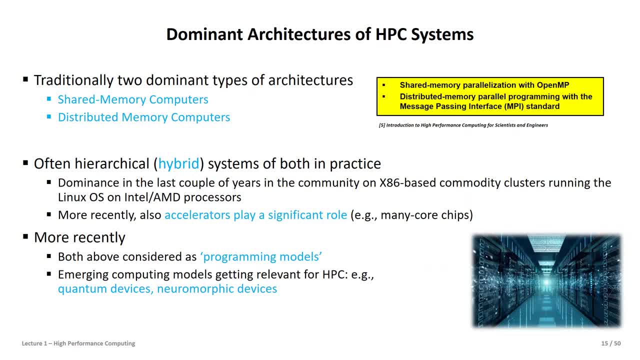 And with this they're kind of two dominant types of architecture- shared memory and distributed memory- And what we see in practice when you go to a whole really, that basically those are more or less hybrid systems And of course, more recently also the accelerators play a much more significant role, as, let's say, 15 years ago. 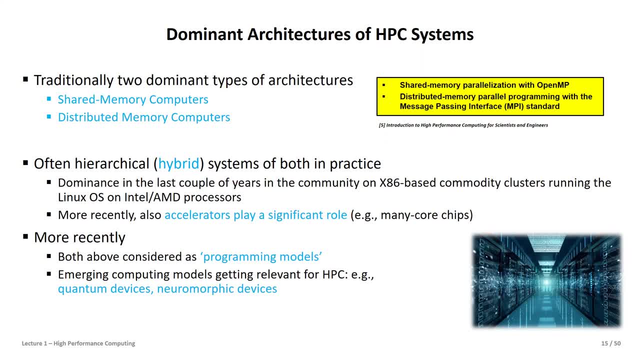 So many core chips, graphics cards and so forth are very important today. So in a way, you would say that shared memory and distributed memory is more or less a view of programming models these days, And we will see also that programming models will evolve. 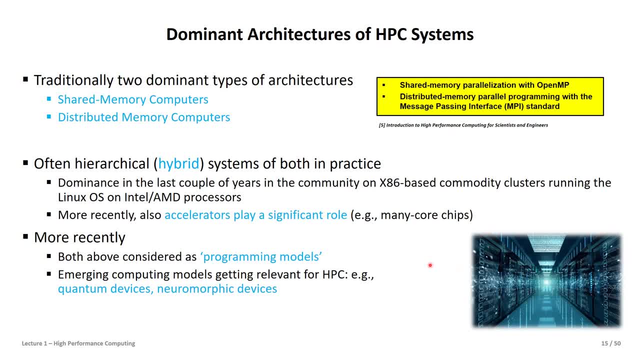 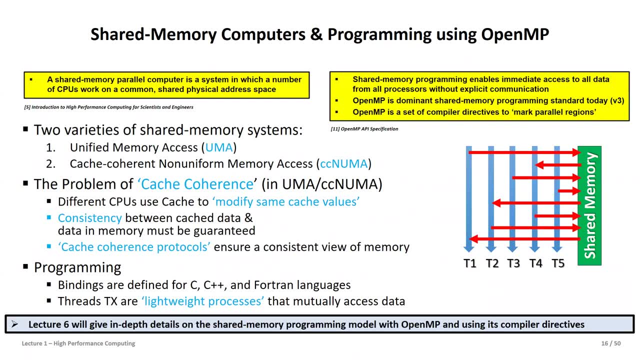 If the future, here at the end of the corridor, we see quantum arising, We see neuromorphic devices, So it's a new form of programming. all of those So for shared memory, and of course, we will have in-depth lectures on this. 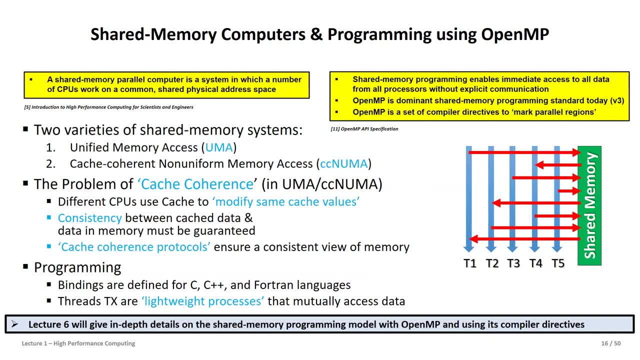 You will program them as part of assignments, But in basically shared memory. you see the idea of basically having always access to your memory, writing, reading variables, And you have different threads that can actually operate on that. Obviously, there's one important language called OpenMP, a standard. 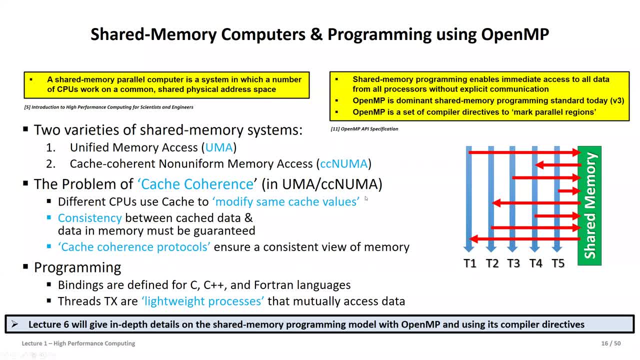 How you basically can program those, And in Lecture 6, we will talk about this. And of course you can imagine you have also some unwanted elements like overwriting variables. We will have to talk about cache currents, levels and so forth. 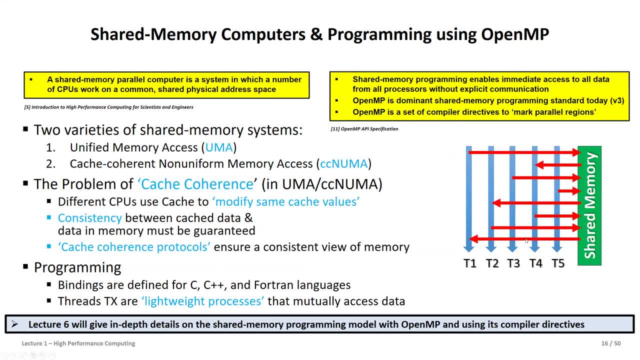 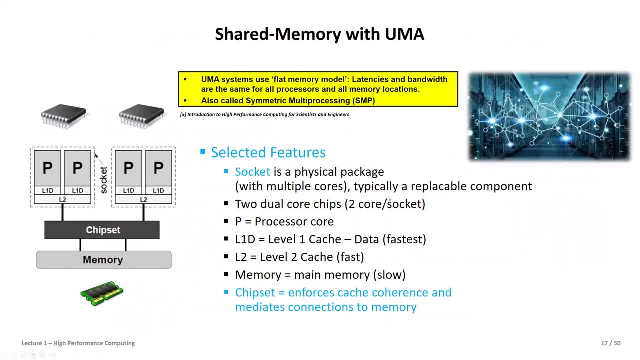 But in the end, the shared memory you talk about lightweight, basically lightweight tools or lightweight threads. So with unified memory access, the shared memory will look essentially like really a flat memory model. So essentially all the same, all the processes are the same. 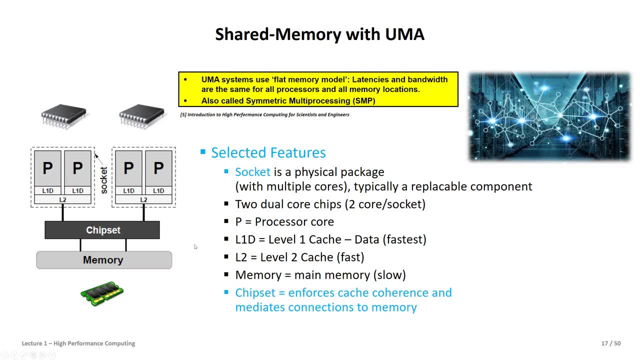 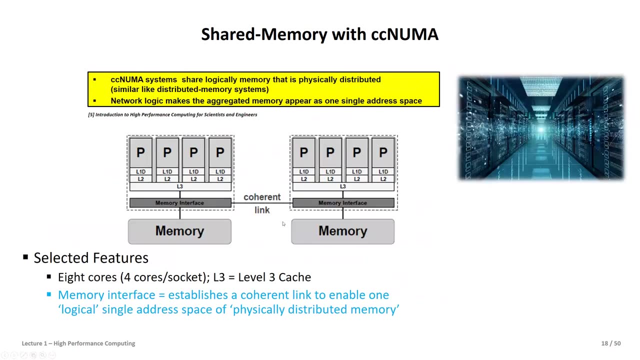 And all the memory locations is also called symmetric multiprocessing. You see that a little bit here. So all have the same way to the memory all these different cores or processes here. So they all have of course their level one caches, level two caches and so forth. 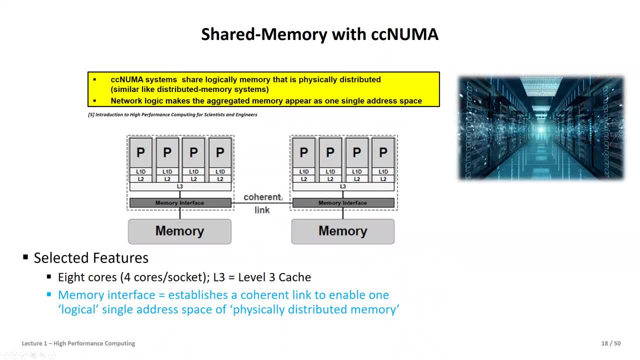 So when you have the CC NUMA, the non-uniform access, you have this cache coherent link. So you see that, essentially in order to go to the other memory, which is a form of distributed memory, but not really, it's still basically logical. 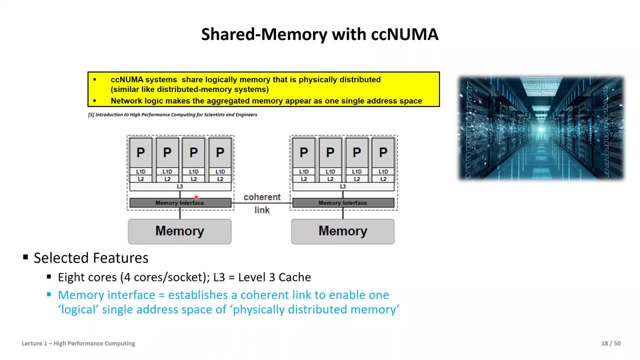 memory that is distributed but still accessible in one logical way. So it's still a shared memory system, But of course here's a protocol that's solving this problem of being distributed, And then you would have a distributed memory which is really now talking. 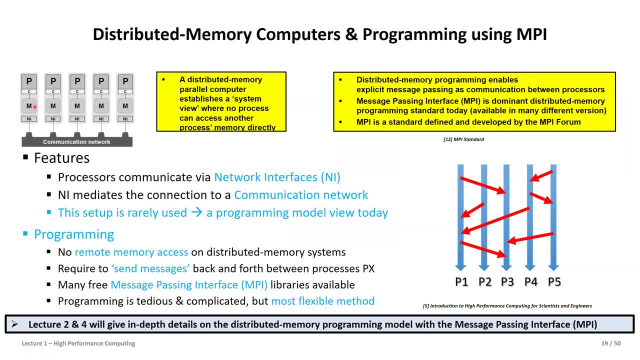 about different processes where there's no way around that you can actually access the other memory. you always have to go to a so-called communication network So you cannot just write and read a memory anymore, and so on. You always have to send messages, And of course this will be a big part in our coming lectures. 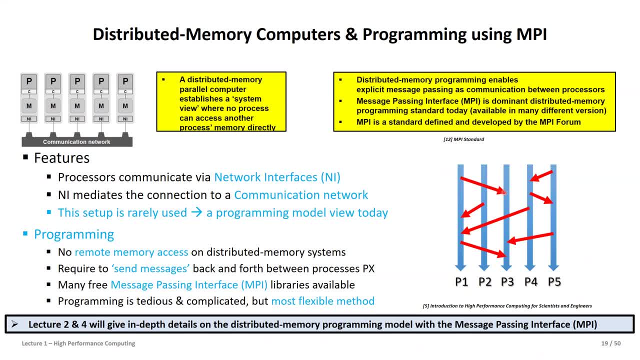 also in your first assignment, to learn what MPI is all about. What means send, receive, what more means reduce, broadcast, the so-called methods, which include, let's say, lots of different processes at the same time, collective operations as we name them. 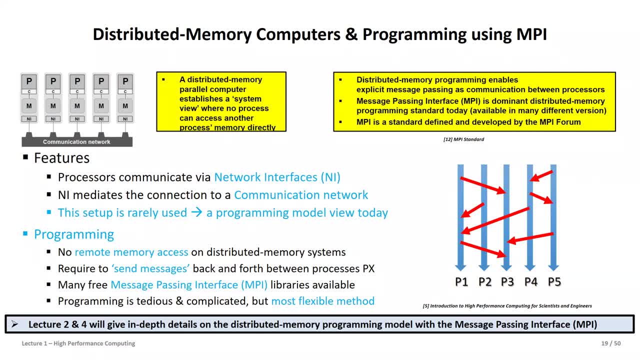 But the MPI is really a kind of de facto standard to program those And we will learn about this a lot in the lecture Two and lecture four. So this is really where we go into the practice very soon And there's an MPI standard that we're going to use. 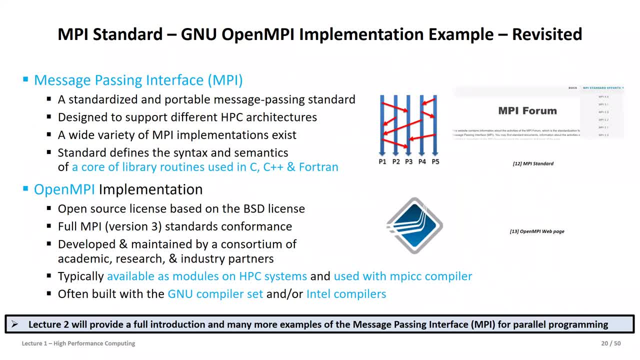 That means many of the code parts you will basically have in front of you will be, let's say, standardized. things like MPI, send, receive. The all API is a standard And, if you want, you can look into this website. You will see the different versions. 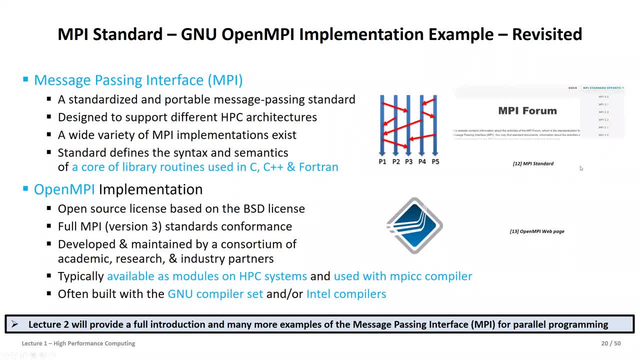 of the standards always being further developed, And for this standard is, of course, important to understand that there is an MPI implementation, And here we talk one specific one, that different ones out there. Here's the open MPI implementation, which is an implementation for the MPI. 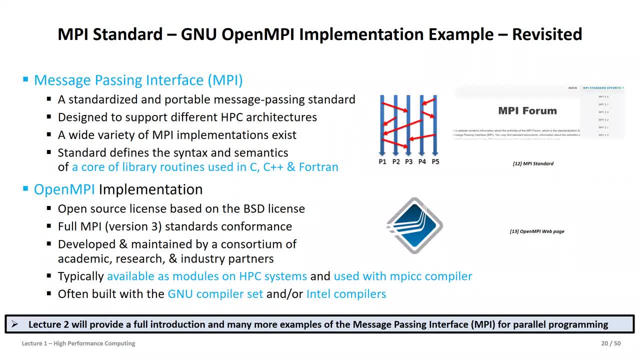 standard that you can then use, maybe in C, in C++, But of course can also use in Fortran, because many of the applications are actually still here and they are running Fortran. But also new applications can use Python, because there's also an MPI for Python. 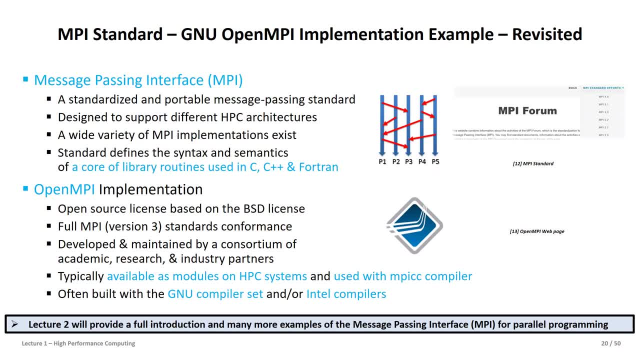 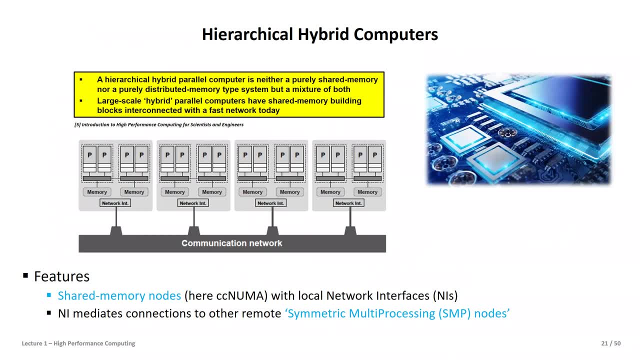 So the standard which has reached really the community standard level in HPC. everybody knows what an MPI code is and it's extensively used. And if you look in the practice how systems are used today, you see hierarchical hybrid computers where basically people program shared memory within the node. 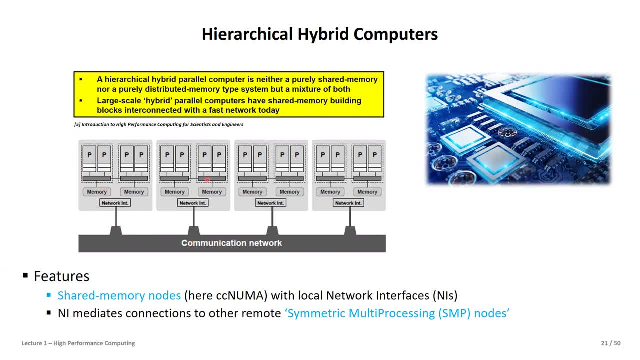 But in order to basically have larger problems solved, you use distributed memory programming And here hybrid. in the end that means you would basically combine the power of the memory systems and program shared memory inside and distribute memory basically across the nodes And you would always have this very good communication interconnect. 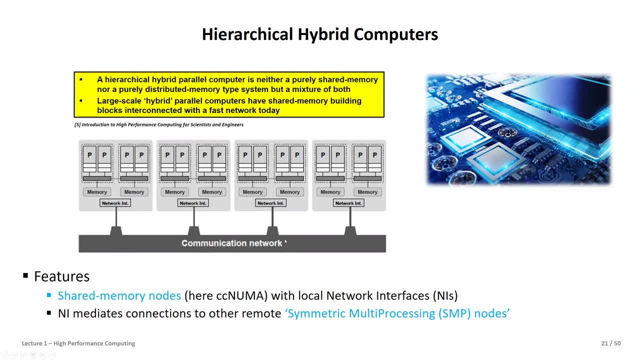 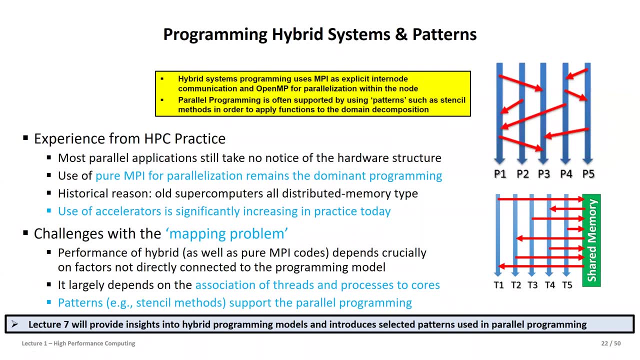 I always was saying in the beginning, which constitutes then HPC. It's usually also the most cost intensive part of HPC machine, this communication network. So it's not easy to actually basically program hybrid. We will have a lecture on this where we will see what. 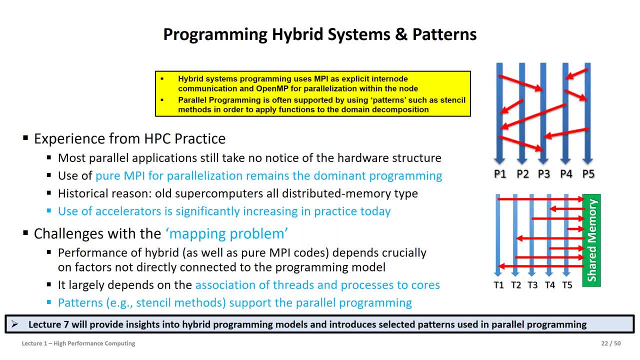 it means really to have these large systems today programmed. If you want to combine shared memory with distributed memory, for example. it gives you maybe here and there the best performance of an application, But on the other hand it's also requires quite some methods. 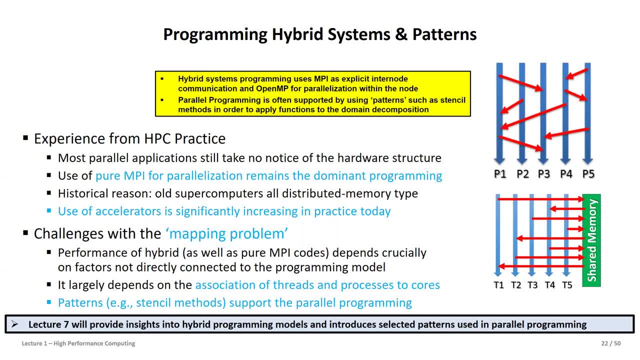 and quite some good understanding what the problem is and basically how you map that really to the technology. But these are things we will talk about in lecture seven, just giving you an indicator of, of course. these days people are combining these different activities. 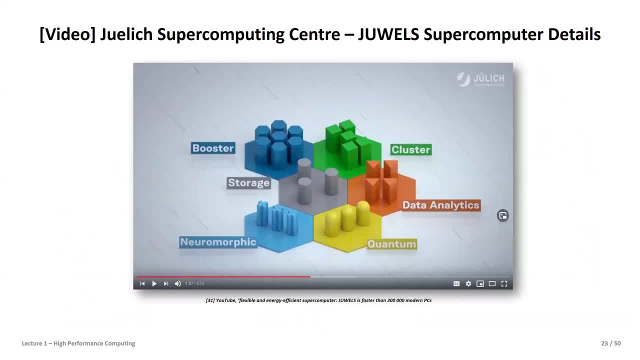 And if, if you want to have more complexity, of course you have to even add the accelerators, And that's something what we deal in. part two. But let us now have a short, basically video here from the Uli Supercomputing Center. that also shows you a little bit what a supercomputer is. 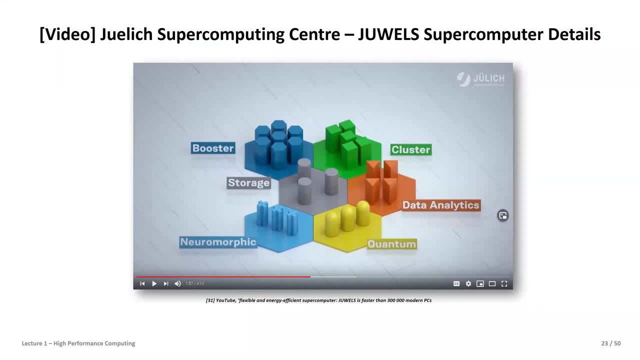 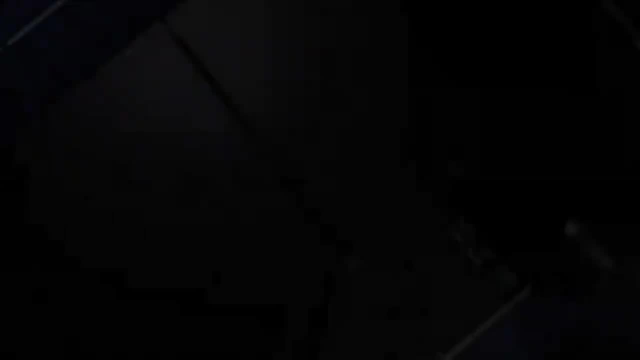 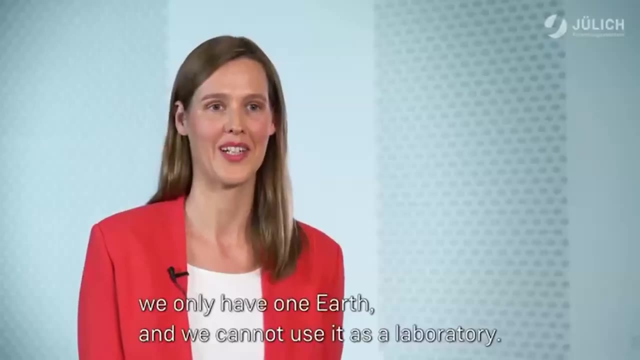 what the modular supercomputing approach is. And here are some, let's say- practical insights. We can't do global experiments here, We only have one earth. we can't use it as a laboratory, But with the simulations we can of course play through everything. 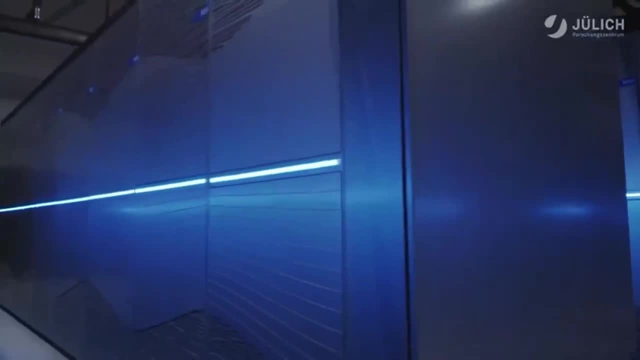 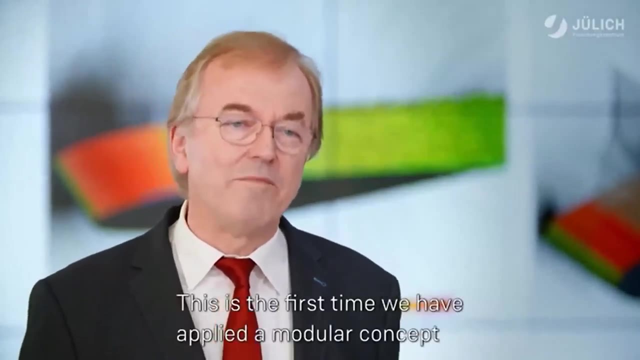 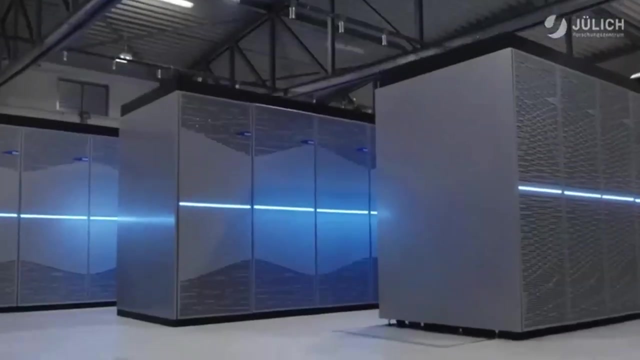 Our supercomputer is really unique. We have applied the modular concept for the first time to a system in this performance class. We have applied the modular concept for the first time to a system in this performance class For some interim. you and its partners have built a supercomputer that is setting. 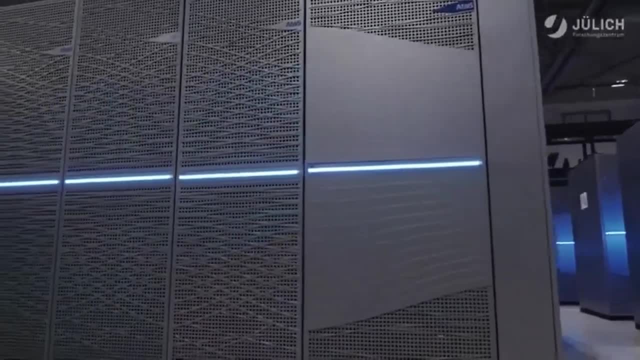 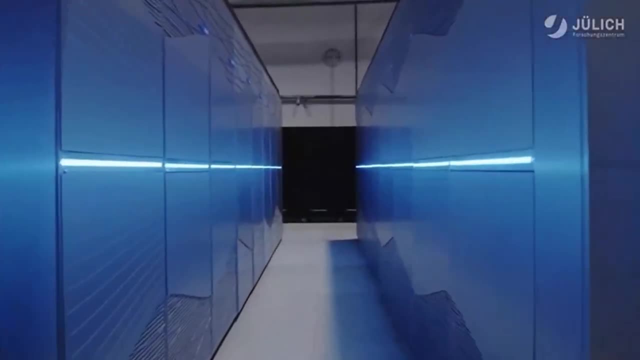 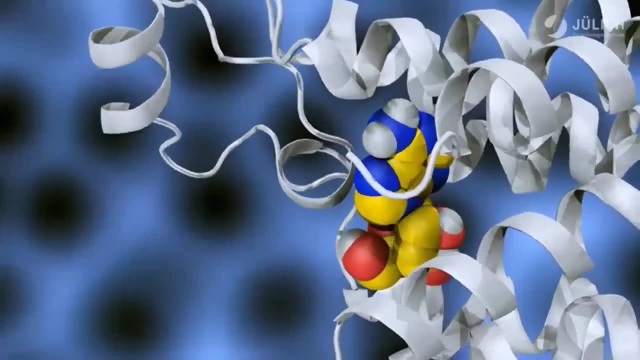 benchmarks on a global scale upon its completion, Jules is the fastest computer in Europe and boasts unparalleled energy efficiency. With its enormous computing power, researchers can accelerate the development of medicines, investigate how the human brain works and clarify whether the process can be on purpose. 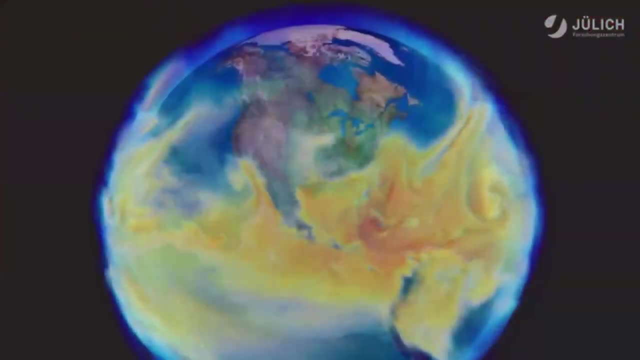 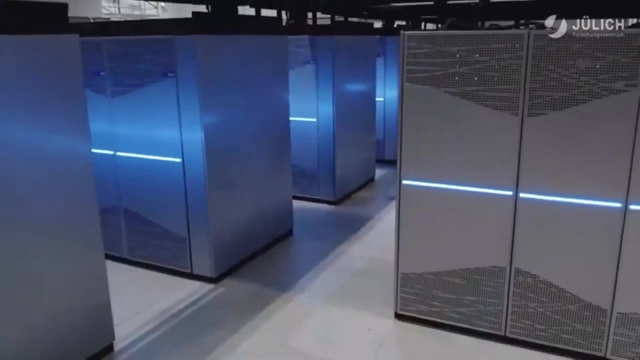 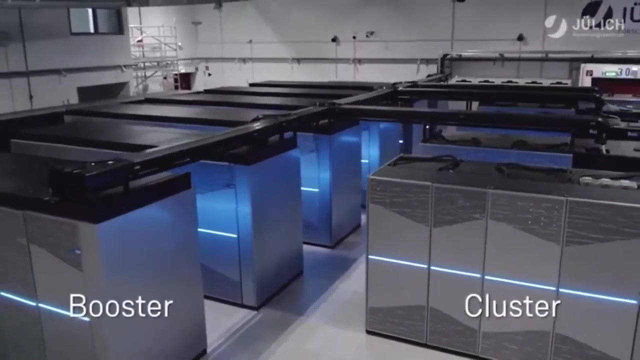 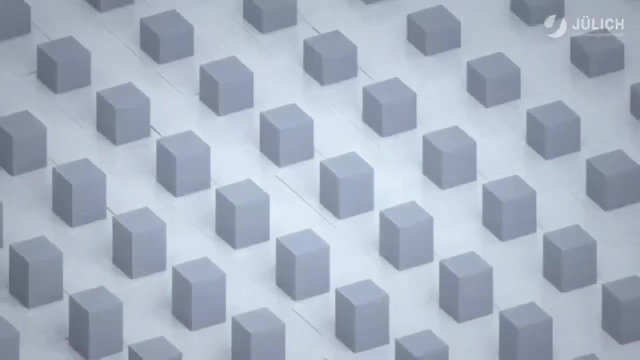 The latest technology in the world, no one knows fundamental questions regarding renewable energy and the climate. crucial to its flexibility is the modular architecture developed at Forsen Zentrum Jülich, comprising a cluster and a booster module which are interconnected in conventional supercomputers. thousands of identical 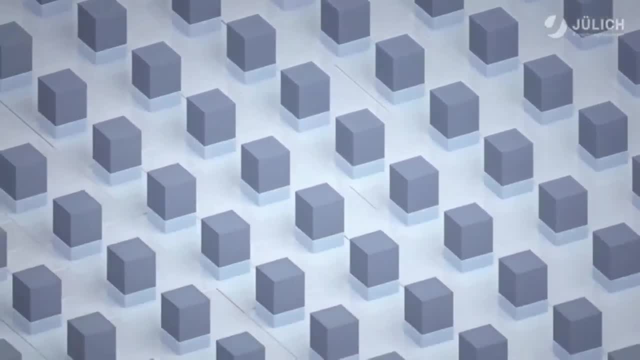 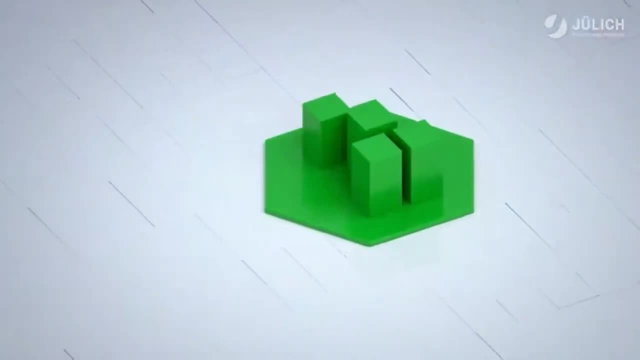 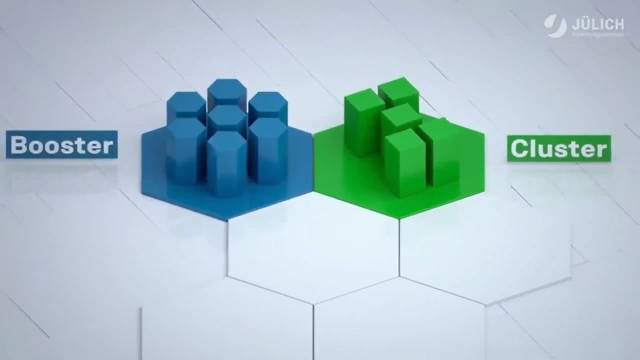 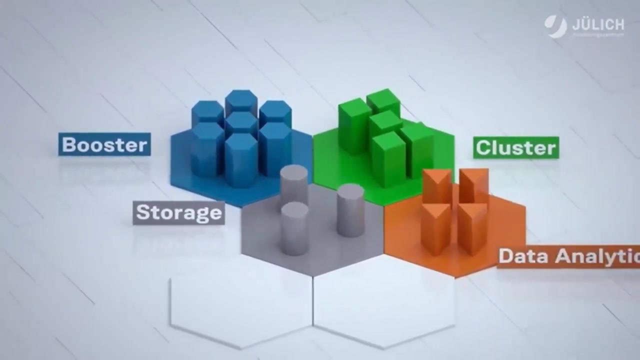 processing units are combined. some applications, however, can only make partial use of them. in contrast, a modular architecture works more efficiently. a universally applicable cluster is enhanced by specialized units, for example in ultra fast booster, a centralized storage system or a module for data analytics and pioneering technologies such as quantum computers.